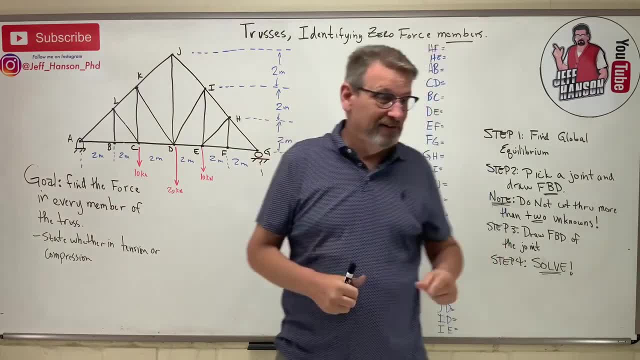 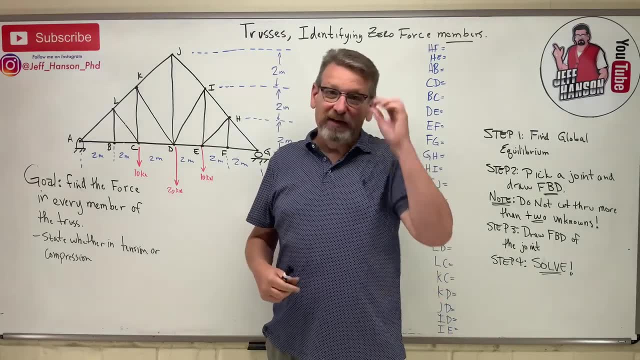 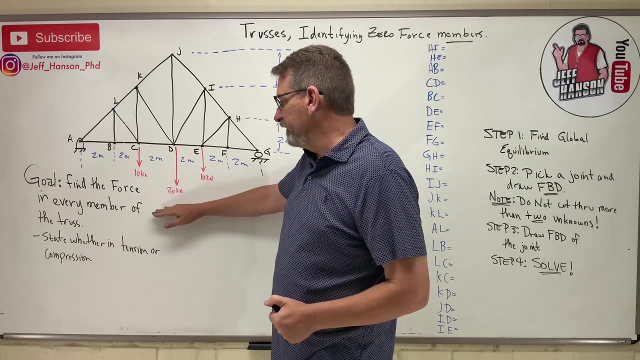 like: oh my gosh, how many members are in this trust? This many, That's 21 members, And we're going to use the method of joints to solve it. I know you're thinking we're going to be here forever. What are you thinking? Okay, So let's look at this. Find every force in the trust and 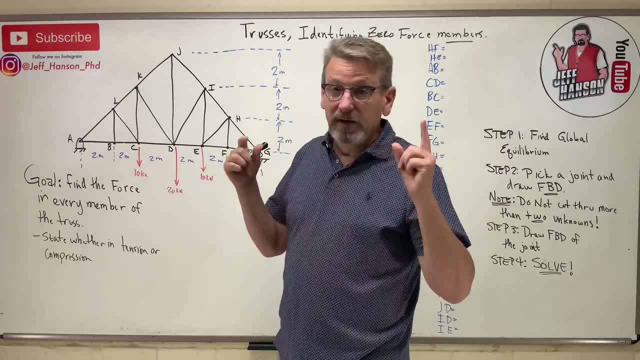 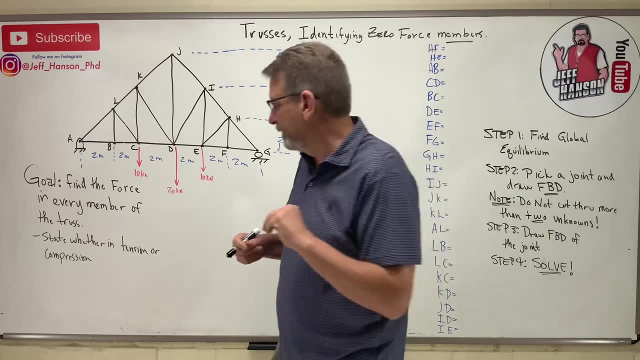 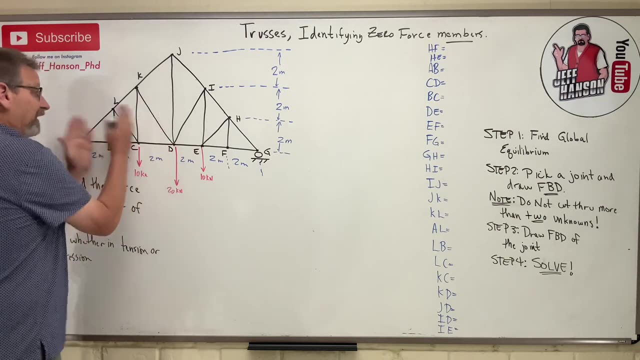 state whether it's in tension or compression. So the same thing we've been doing, But first. well, there's a couple of things to identify. This is a little bit simpler problem right off the bat. Number one: Okay, Things you should be looking for. Number one: this is a symmetric trust. The left side is 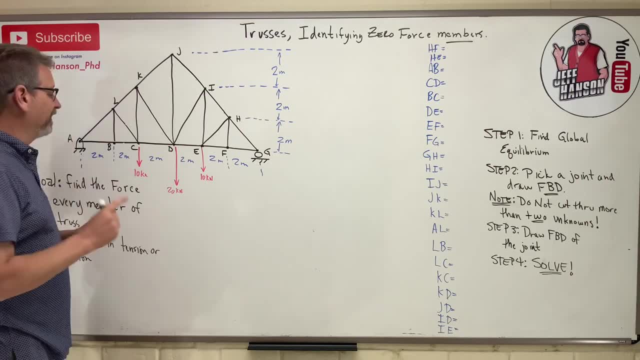 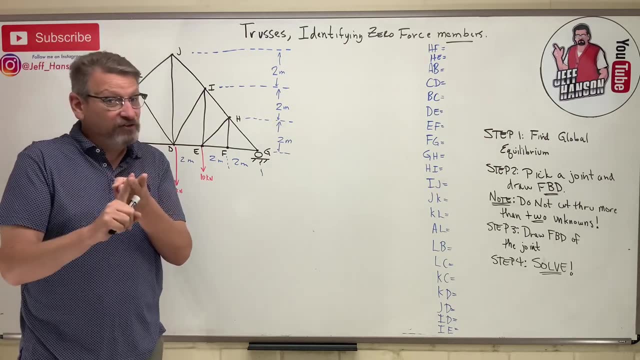 the same as the right side. Also, in addition to that, it's a symmetric load right: 10,, 20,, 10.. So if you have a symmetric trust and a symmetric load, you have to have both of those. But if you 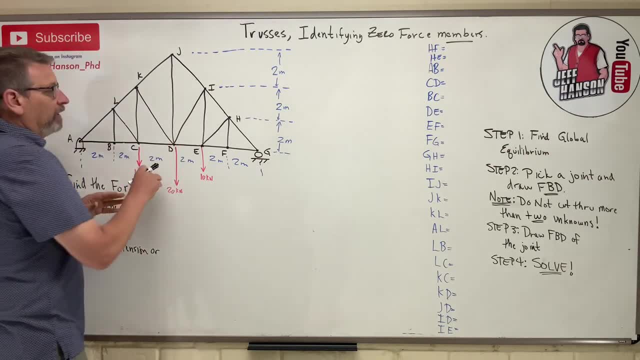 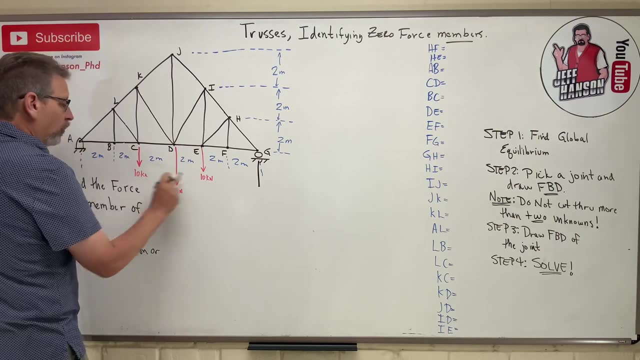 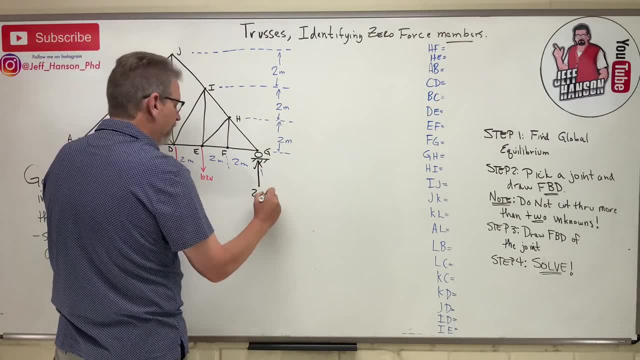 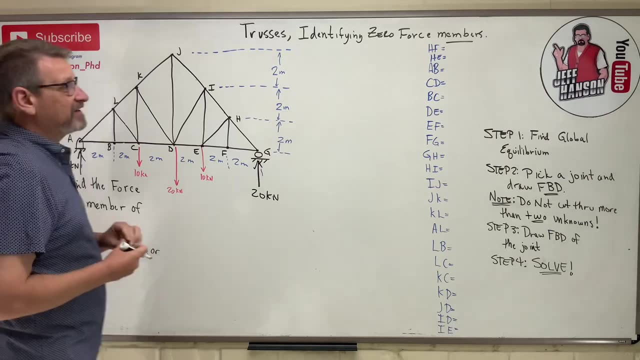 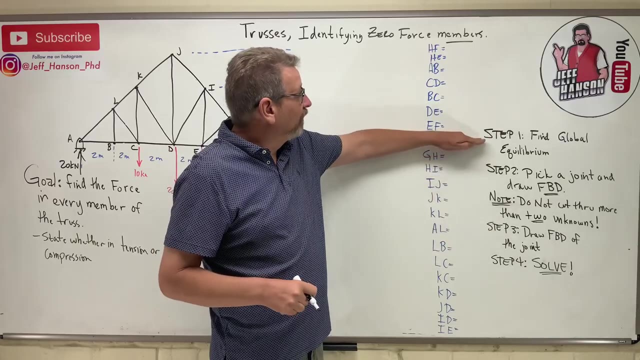 plus 20 is 40.. So you get 20.. Okay, Kilonewtons, And you get 20.. And there is step one. You'll remember this little recipe over here from our discussion on the method of joints: Define global equilibrium. Well, guess what Done. Okay, Step one done. Now it says pick. 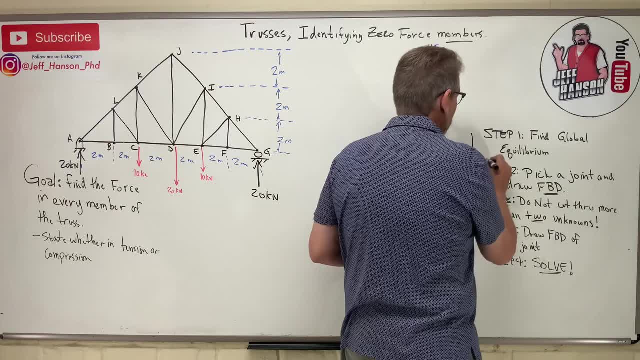 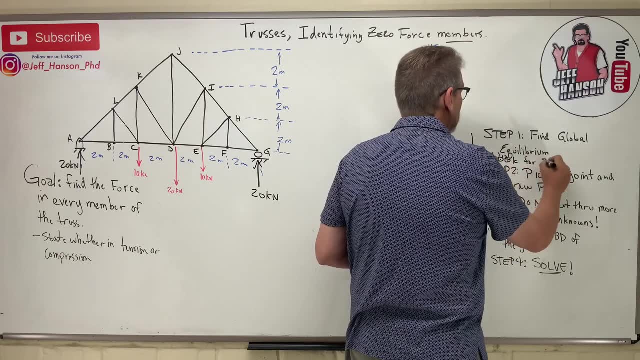 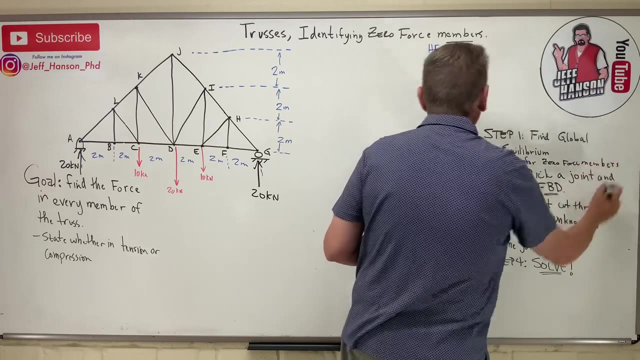 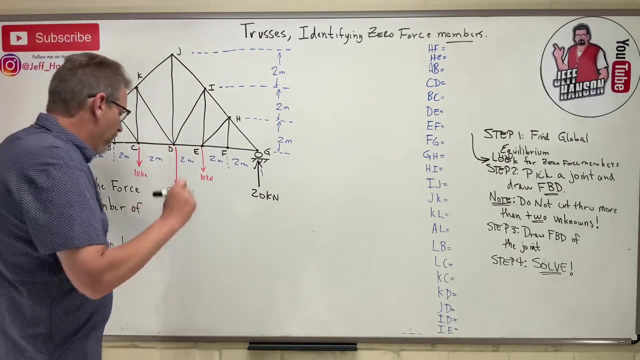 a joint here. but really there ought to be a sub step in here that says: look, Okay, Those are eyeballs. Look for zero force members. Okay, Well, what's a zero force member? Okay, You got to do some little mental freebinding diagrams in your head. but here you go Anytime that you have two. 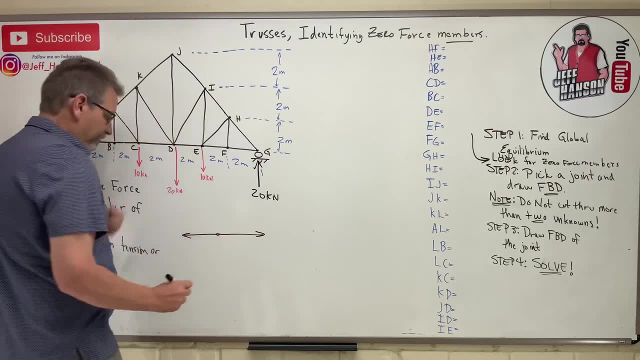 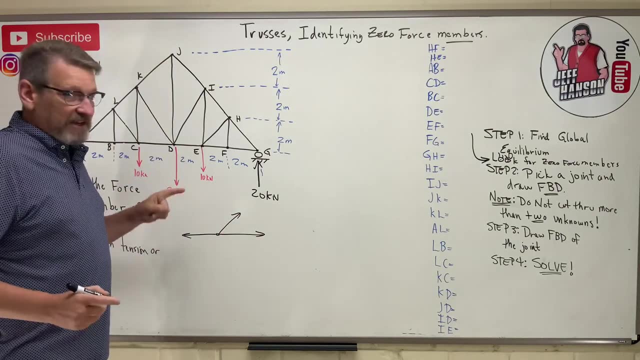 forces, okay, that are on the same line of action and you have a third force that goes like that. let's say right, And just think about this: Something to the left in the X, something right in the X, This guy has. 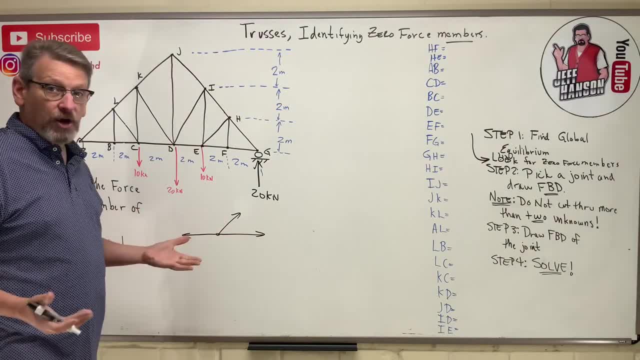 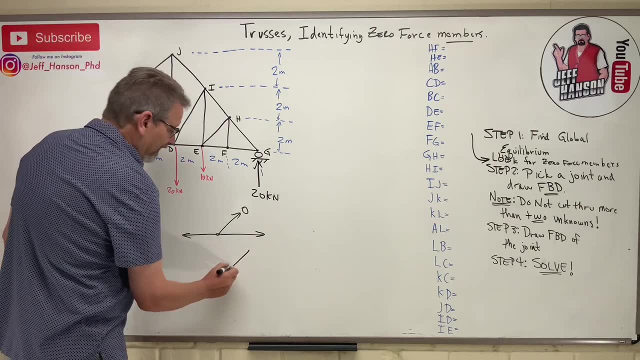 a Y component. Who else has a Y component? Nobody. So guess what? This guy has to be zero, Has to be Okay, And it doesn't matter if he's like that or if he's like this, right, Because some people say: 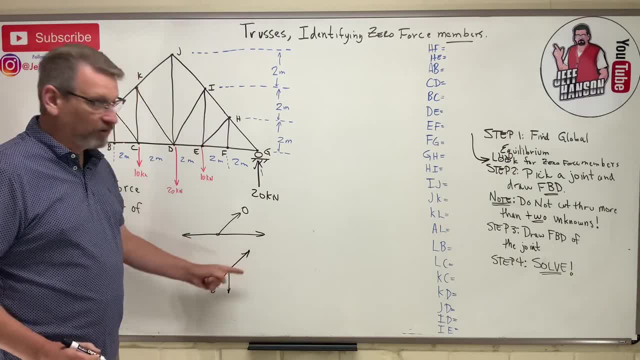 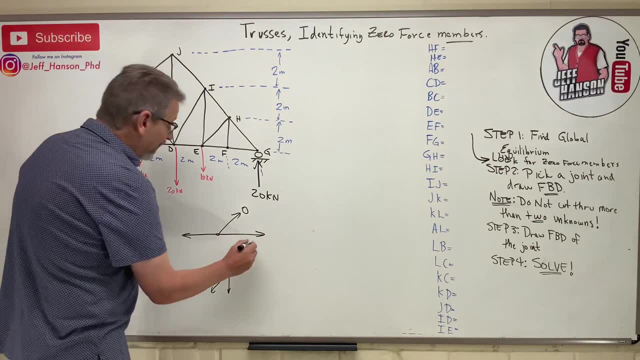 oh, I got something going up, I got something going down, I got something going left, I got something going right. I don't know if he's zero or not. Well, just take that guy and spin it. It's this Okay. So anytime you have two forces that are on the same line of action, and you have 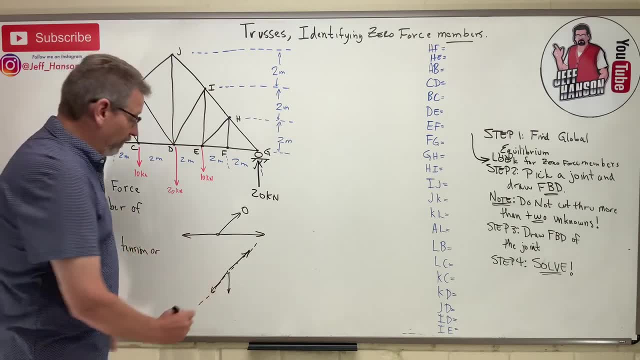 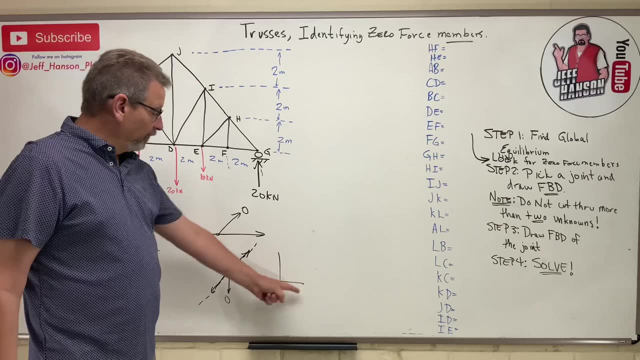 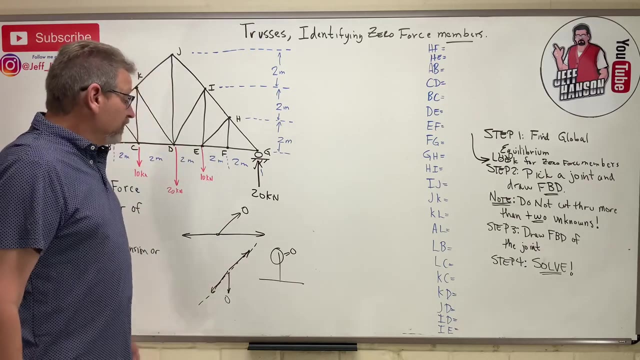 a third one. the third one is always zero. Always, The easiest ones to identify are the ones that look like a T right. If you have some of the left, some of the right, something up but nothing down, then this guy has got to be equal to zero, Just has to be. Okay. So zero force members. 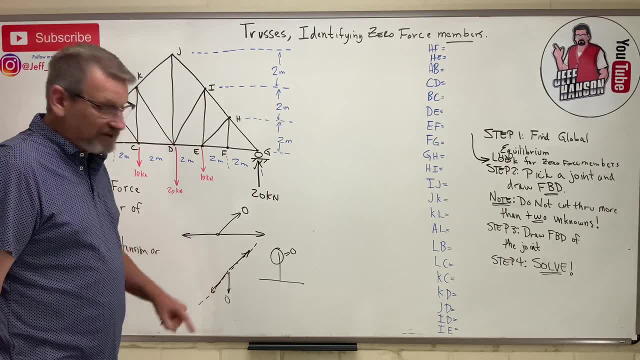 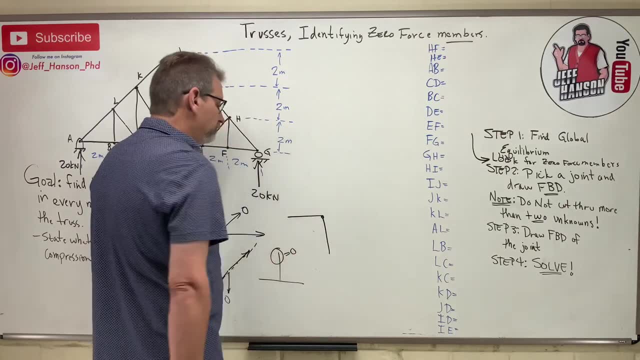 pretty easy to identify in that if you have two on the same line of action. third one is zero, always Okay. There's one more case and that would be like this: Let's say I had a joint like that, Okay, Well, look here I got something to the left, nothing to the right. 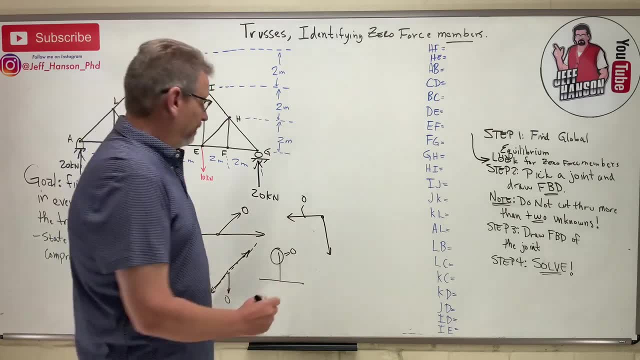 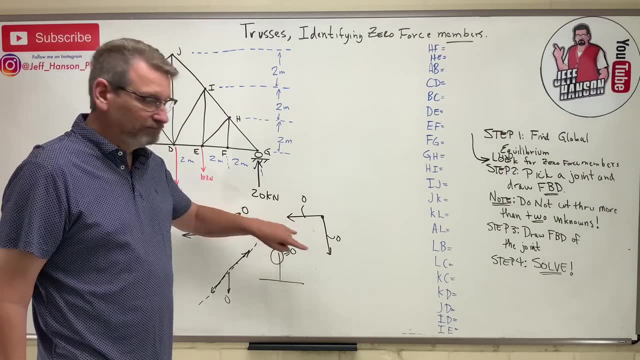 This guy is zero. I got something down but nothing up. That guy is zero. So anytime you have a free body diagram with only two members on it that are not on the same line of action, they're both zero. They got to be Okay. So that's how we identify zero force members. 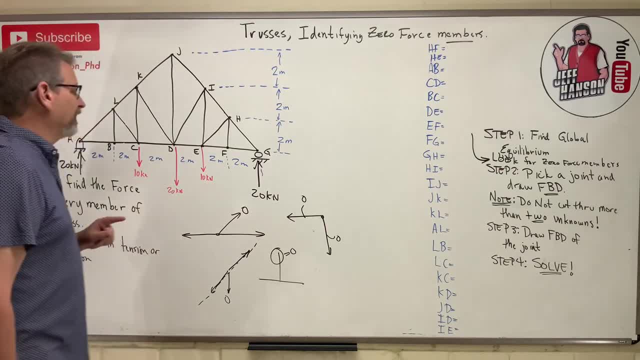 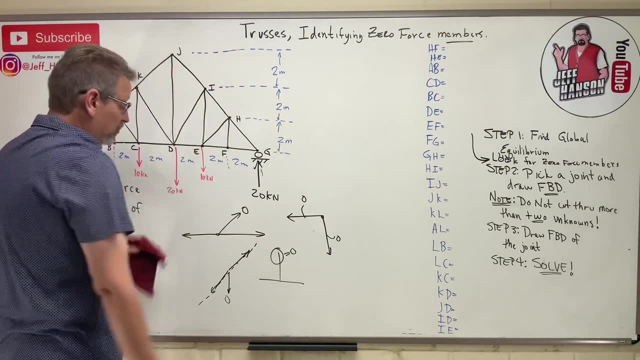 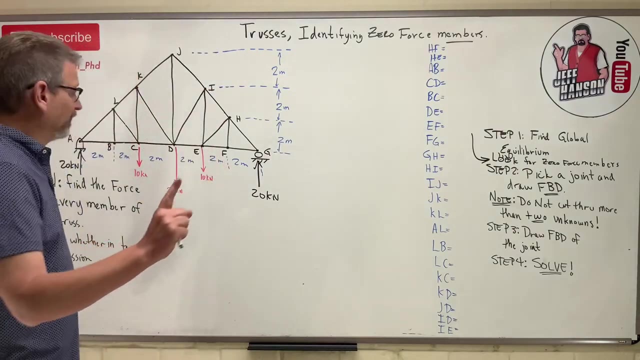 and identifying them, All right. So let's see if we can, let's see if we can simplify this trust, because that right, there is scaring me. That's 21 members in this trust, 21.. Well, but number one is that, since 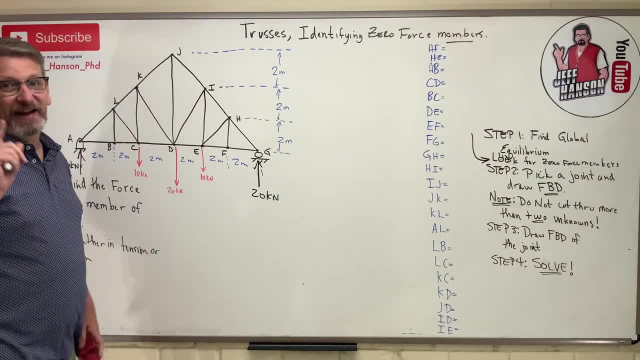 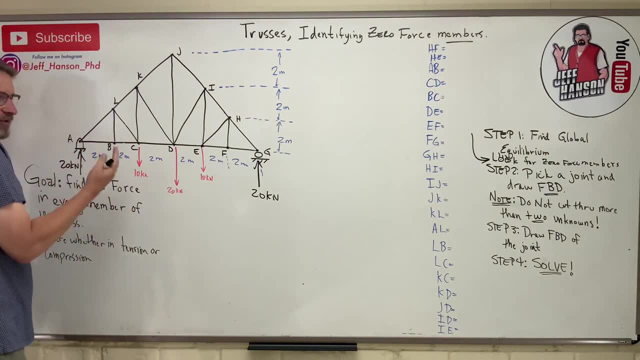 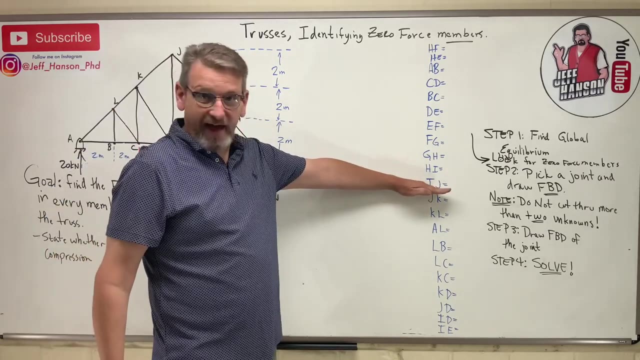 this is symmetric, that already. that already cut my work in half, because whatever's going on in member HG is going to be going on in, AL right? So if I find something on this side, then I automatically find it On that side, right? So right there, boom, I just cut our list in half. Okay, So that. 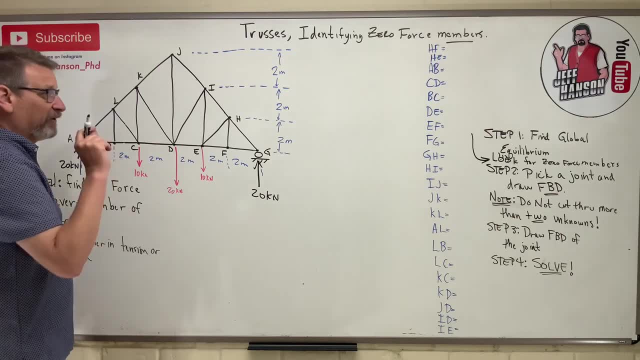 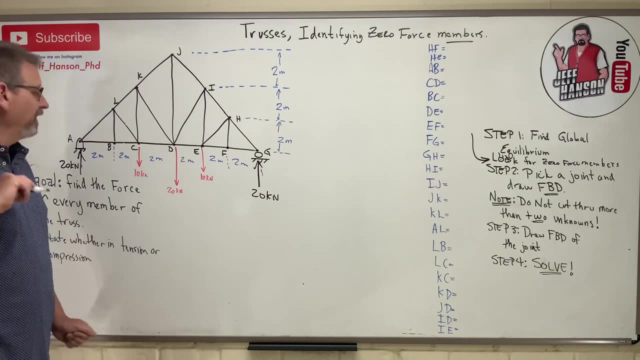 so don't be, don't be panicking anymore. Okay, Let's see if we can find any zero force members in here. Okay, Do you see any? All right, What do you see, Tell me? Okay, All right, I heard you. 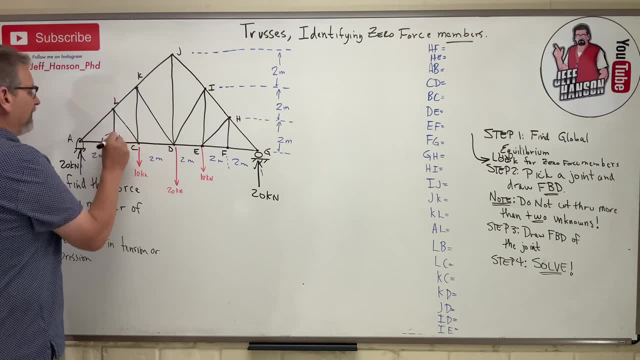 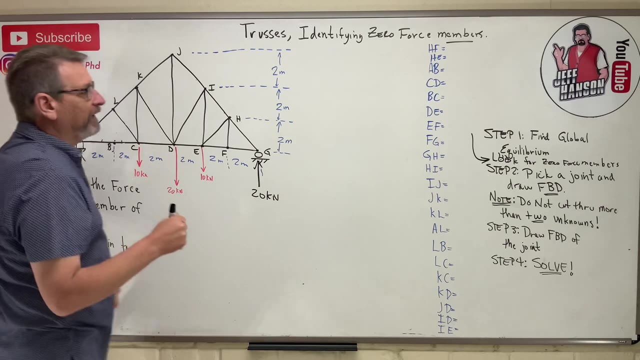 say BL, right. If you look at this free body diagram right here, BL, right. I got something to the left, something to the right, something up but nothing down. So BL is a zero force member. We can take him away. Okay, Take him away. So BL, BL. where's BL, BL, Where? 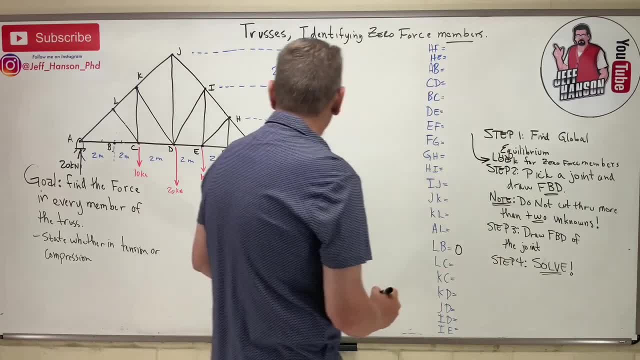 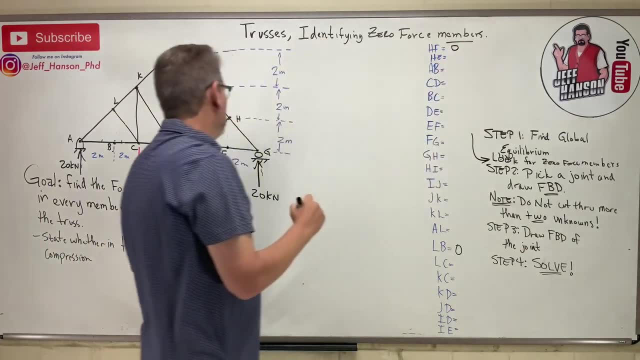 is BL There he is, He's LB. He's zero. Okay, Oh, and so is HF HF zero, Way up there at the top. Okay, Ooh, ooh, look what it did. Now look, I got two fourth, two members on. 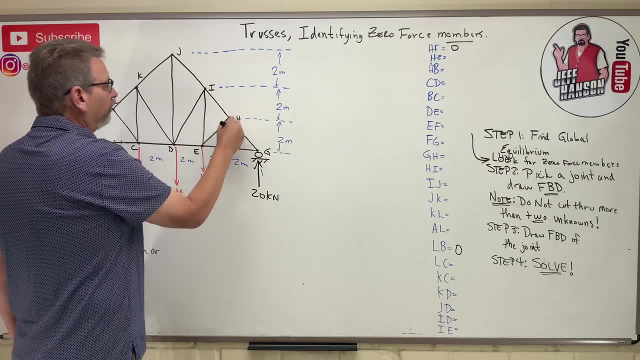 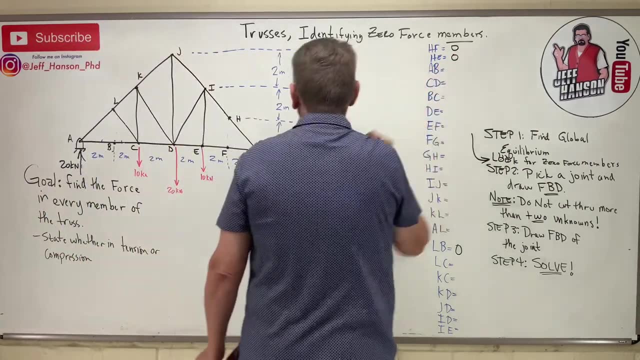 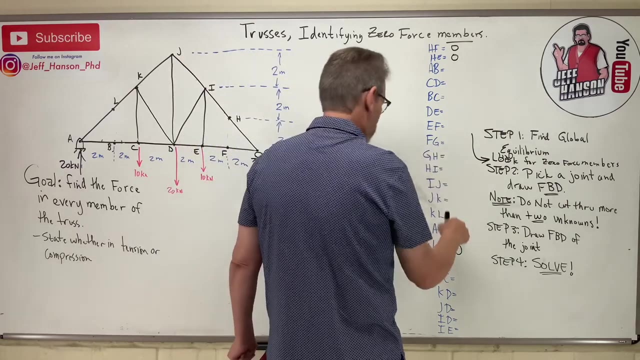 the same line of action and another one. right, If I do a free body diagram, I'm going to do a free body diagram of my head, of that joint. So HE is zero, HE, zero. Okay, Also, LC, zero, LC. where are you LC There? he is, Okay, Zero. So right there I have made. 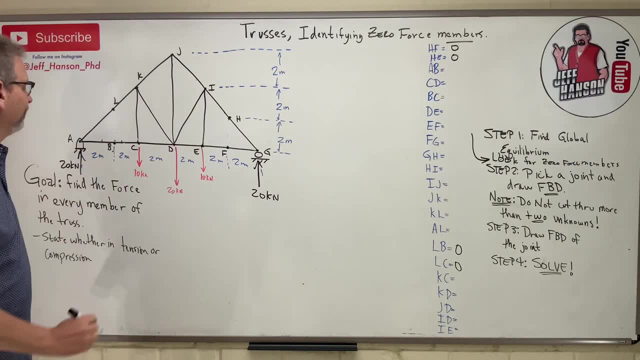 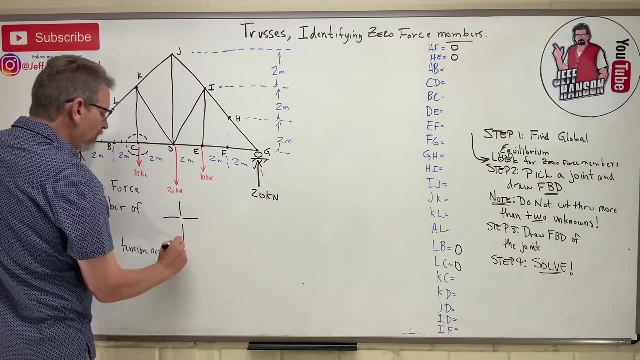 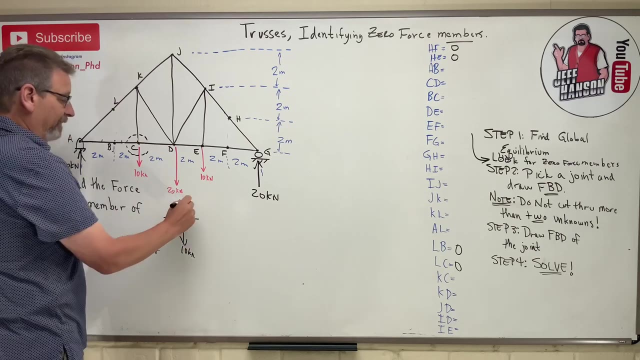 my life a little bit easier. Okay, Now there's a couple other things that are easy. If I look at this one right here, okay, if I look at that joint, I have something like this: Well, I got 10 going down, So what does that guy have to be? Bam, 10 going up, Got to be. 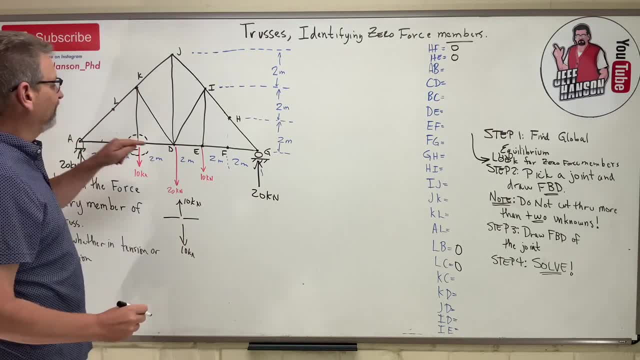 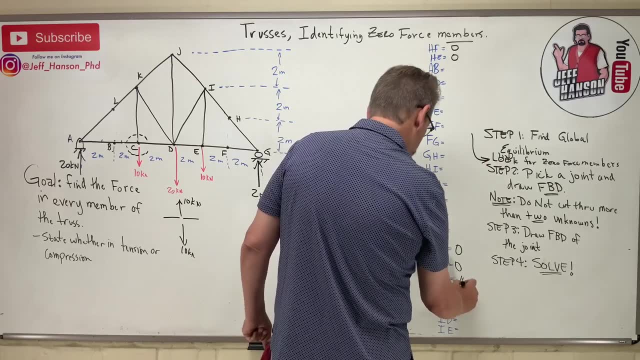 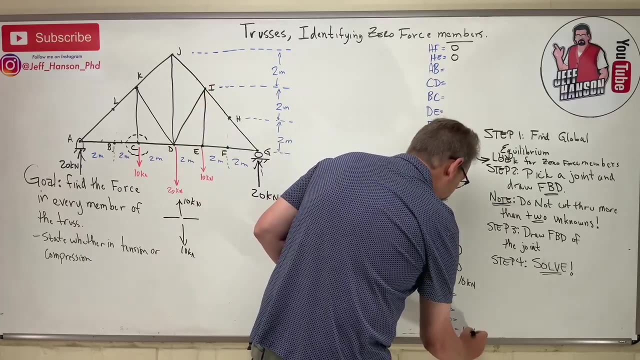 right. So guess what? CK is 10 and EI is 10.. CK, CK. where are you CK? There you are 10 kilonewtons. And what else did I say? IE, That's down at the very bottom. Okay, And that guy is. 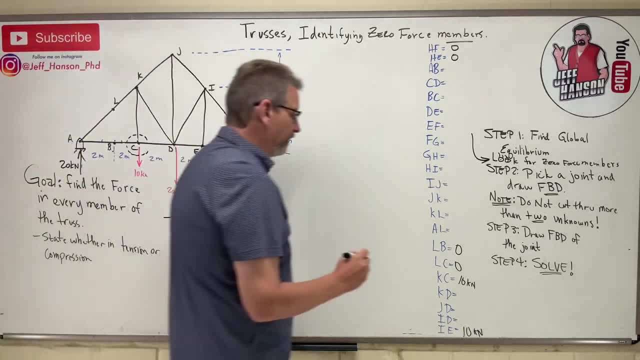 going up, IE is down at the very bottom, Okay. And that guy is going up, IE is down at the very bottom, Away from the joint. So what is he Tension? So this guy's tension, That guy's tension, Okay. 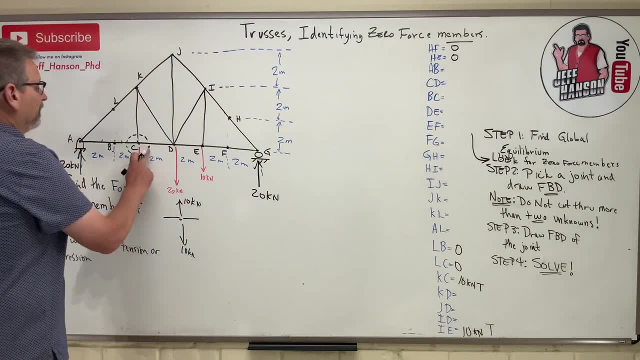 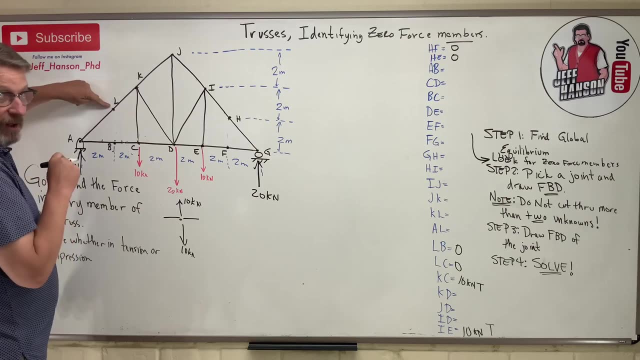 Wow, Look how many. we already got a bunch done, don't we? Okay, Okay. Now here's another thing that makes this easy. If you drew a free body diagram of joint L, now, right, Right, If I draw, 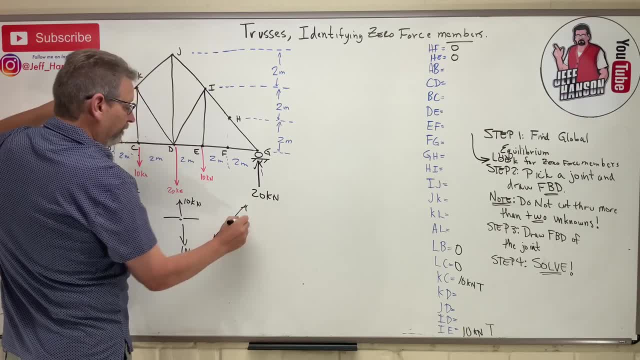 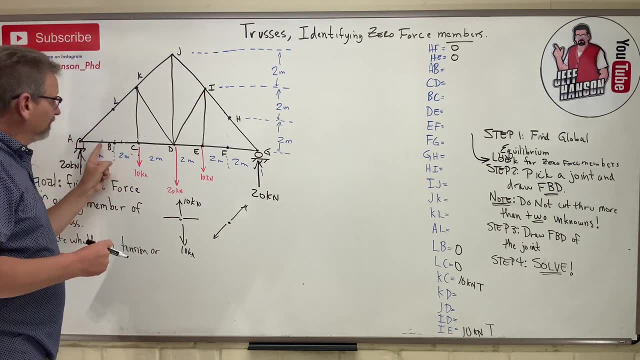 a diagram of joint L. I've got this which tells me that AL and LK- they got to be equal. So does AB and BC and CD, right? So that is equal to that is equal to that. They're all the same. 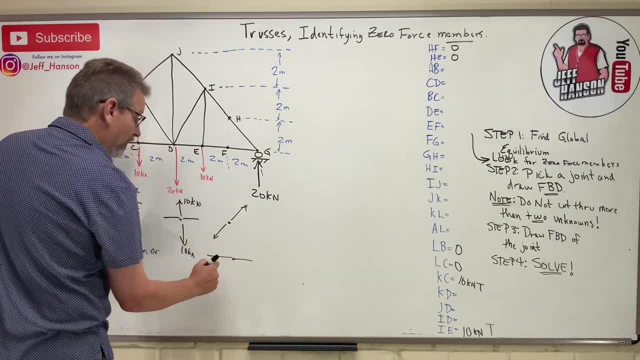 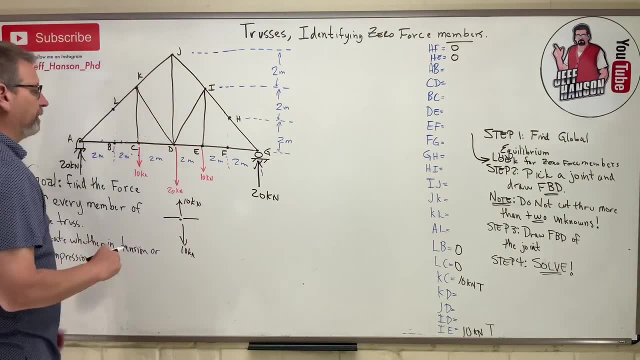 right, Because the free body diagrams like this of the joint, right? So whatever's on this side, it's got to be the same on that side, right? So this is going to be okay. We're going to simplify this quite a bit here. Let's just do a couple of joints and we're going to be there. Okay, Let's. 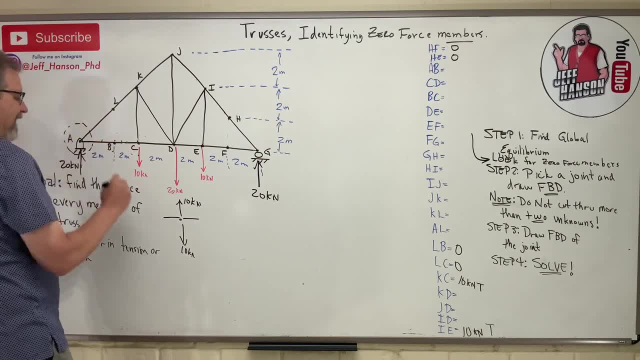 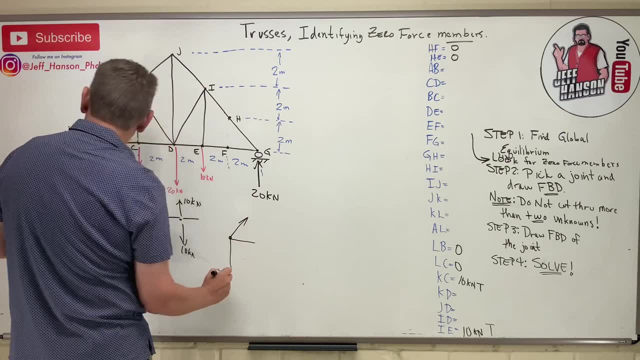 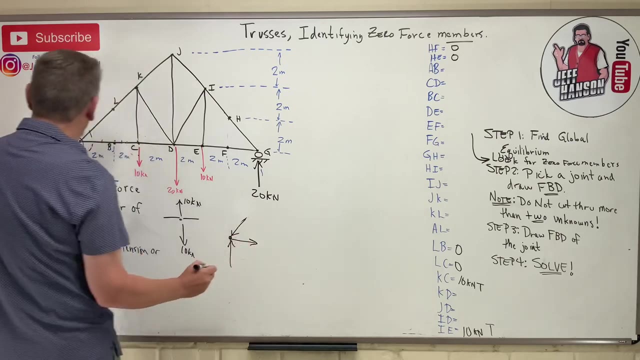 do joint A. So I'm going to do a free body diagram of joint A. Okay, Joint A looks like that. Let's see, This is going up. Oh, this one's got to go down, doesn't it? And if this one goes to the left, then this one has to go to the right. Okay, So this is AB. 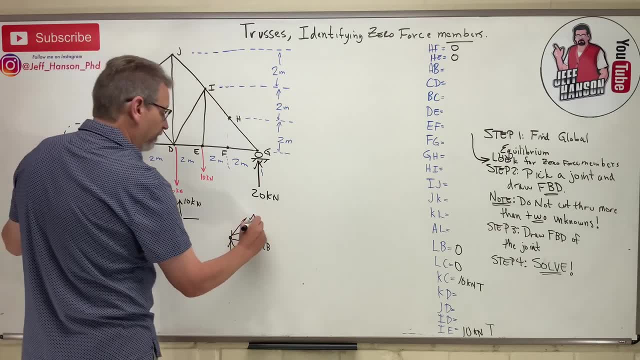 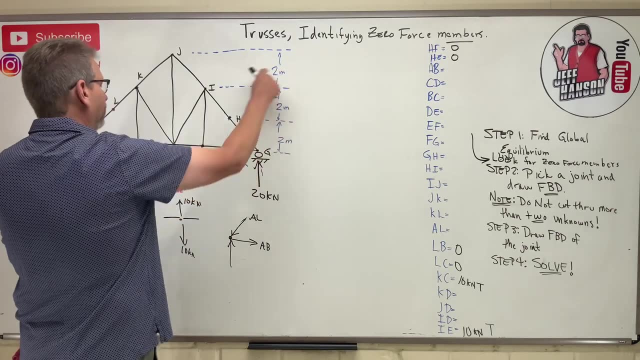 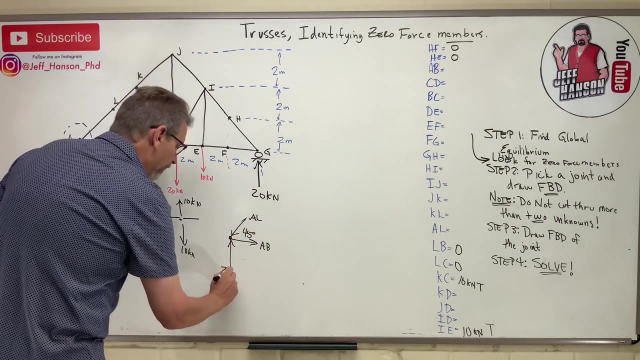 and this guy is AL And the angle is two four, six by two four six, Oh, it's 45 degrees, Okay, And this is 20 kilograms down here. Okay, So quickly I can do the sum of the. 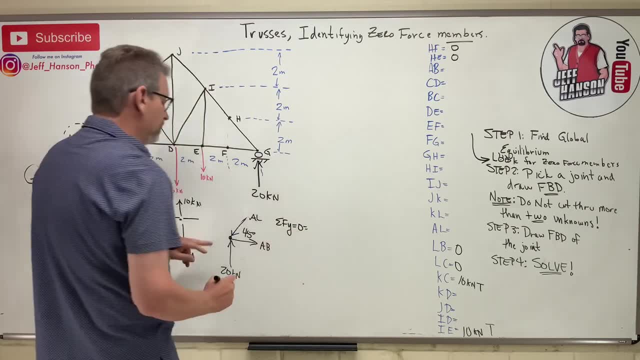 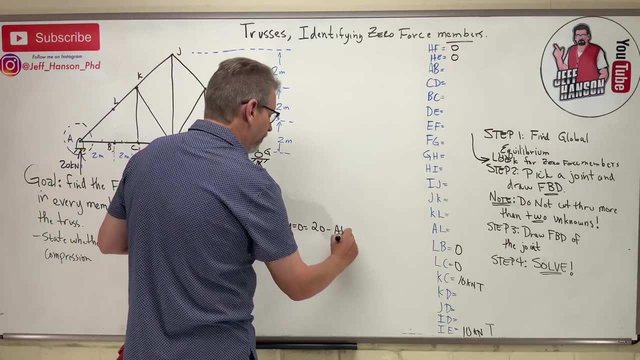 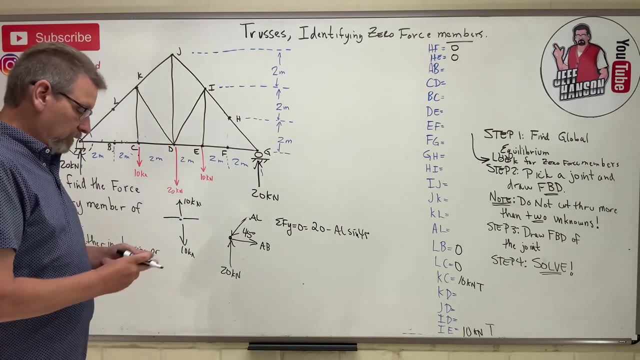 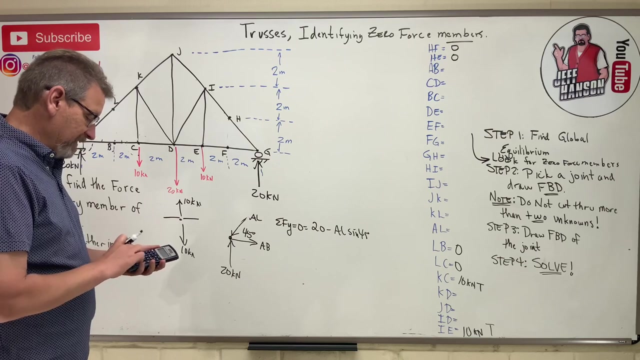 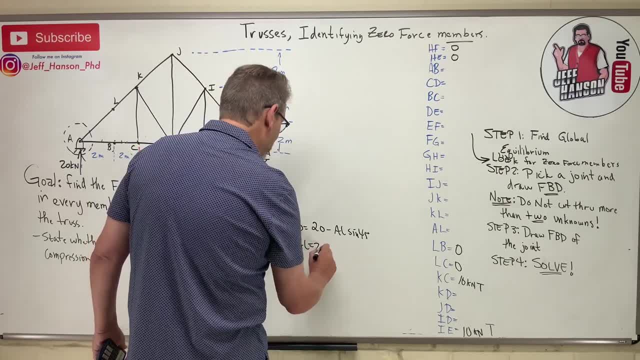 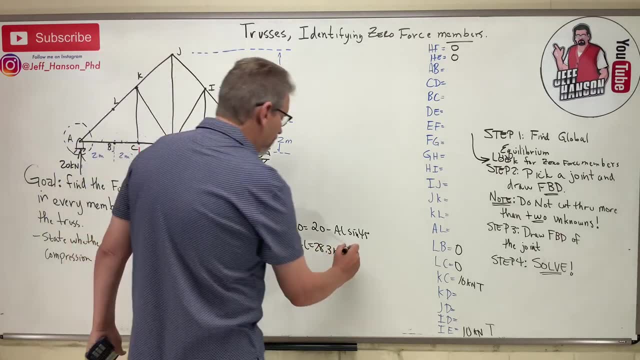 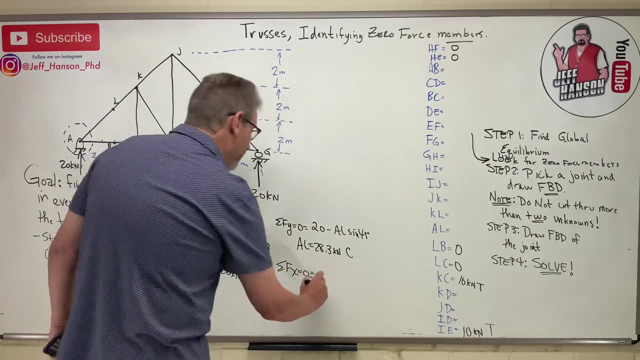 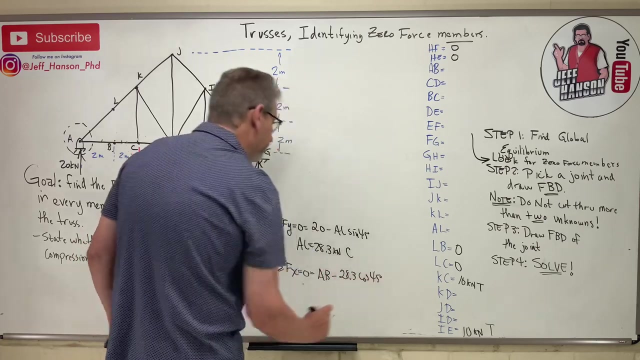 28.3.. So AL equals 28.3 kilonewtons And what It's pushing on the joint. So that guy is compression, Okay, And then I can do the sum of the forces in the X and I get AB minus 28.3, cosine 45. Right, And what is that? 28.3 times 0.707 equals. 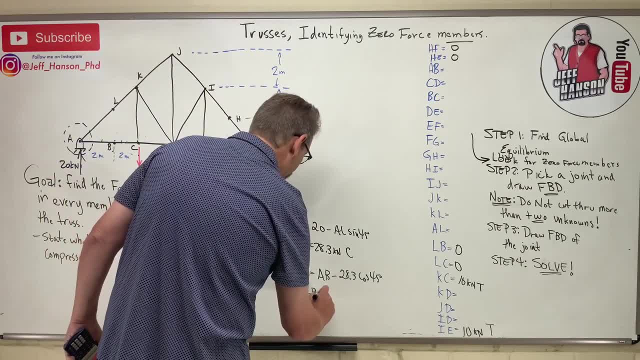 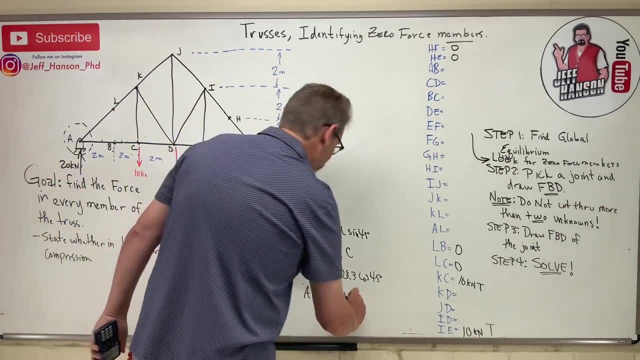 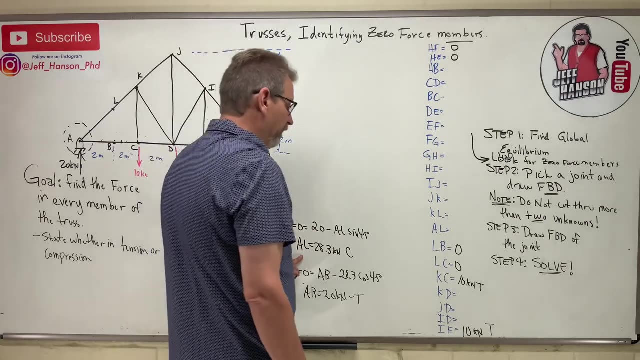 Well, that's 20.. AB is 20. And AB is pulling on the joint, So he is in tension. Okay, So let's put that over there. AL 28.3.. AL, where are you There? you are 28.3. 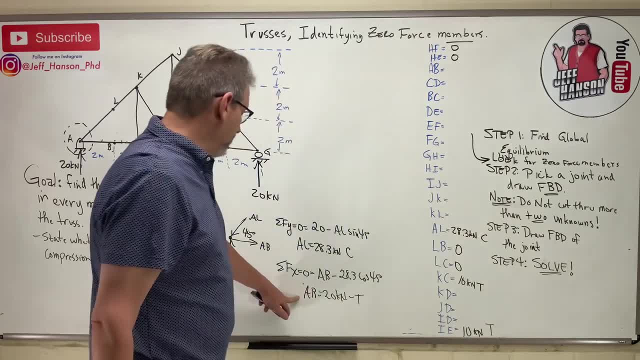 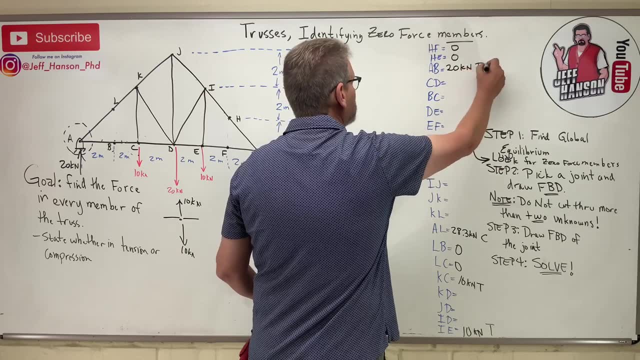 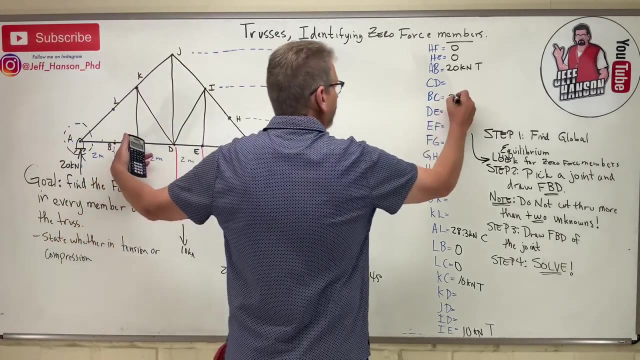 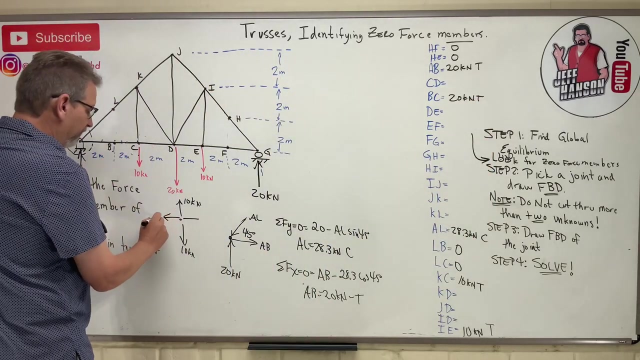 in compression And then AB is 20 kilonewtons. AB is way up here, 20 kilonewtons in tension, Okay, And that means that BC is 20 kilonewtons in tension And that means that CD right, Here's BC, Here's BC And then here's CD. 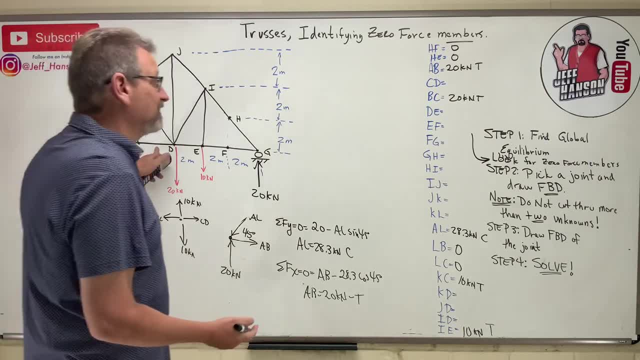 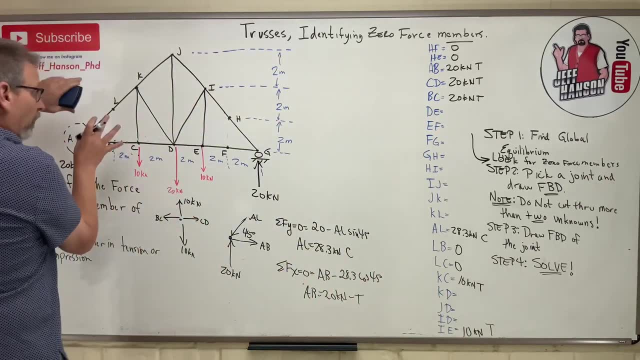 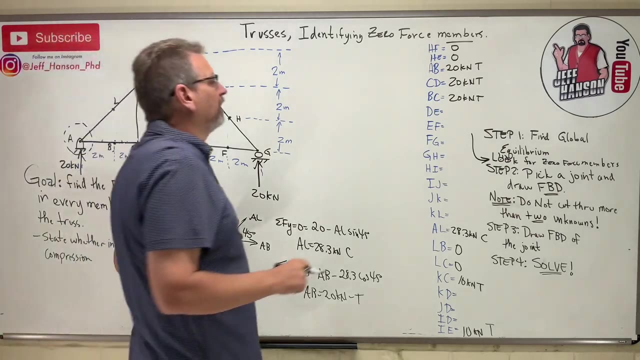 Right. So guess what? He's got to be the same. So CD is 20 kilonewtons in tension. And also, you know what we had over here that we just found? Oh yeah, we can do LK, right? LK has to be the same as AL, right? Where's LK? LK right there. So that one is the 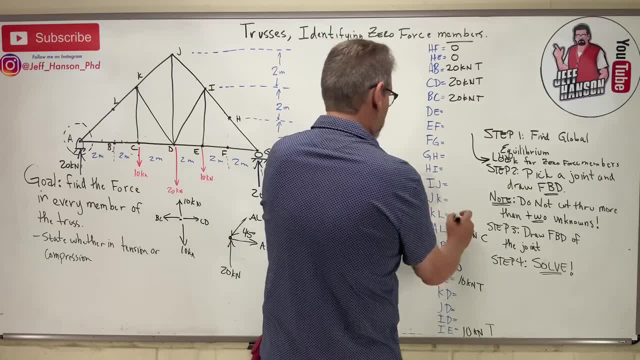 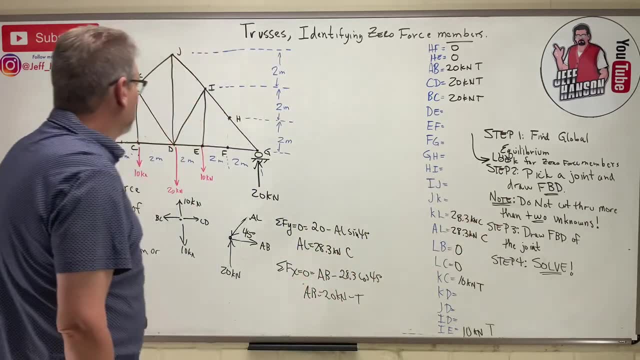 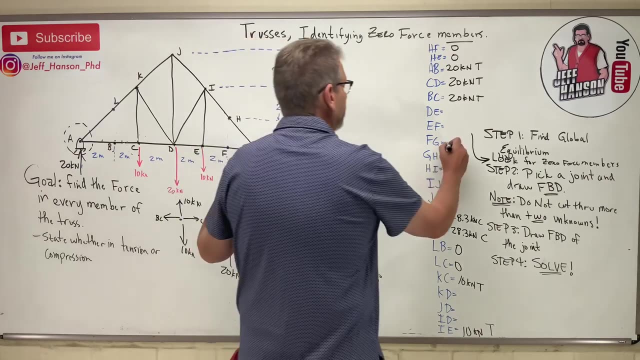 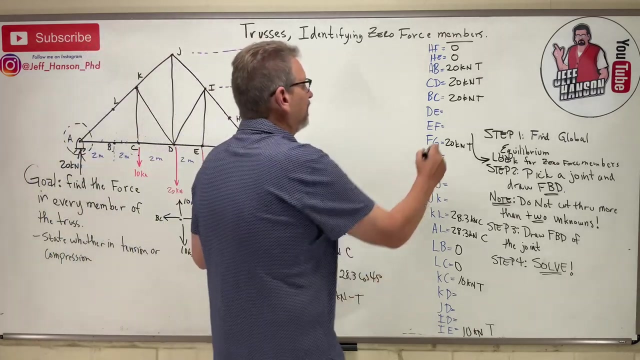 same as AL, which is right there. This one's 28.3 kilonewtons compression, And then these are in tension over here, So GF is 20.. All right, And so is EF and DE, So all these are 20.. 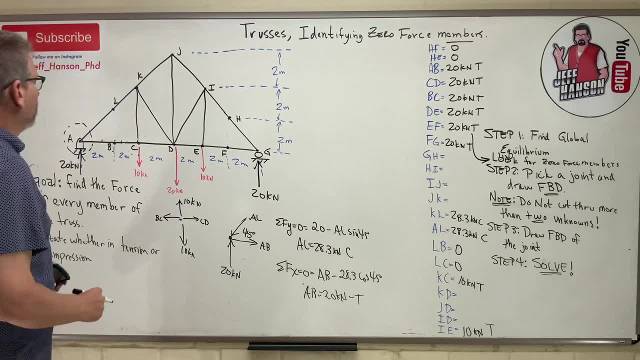 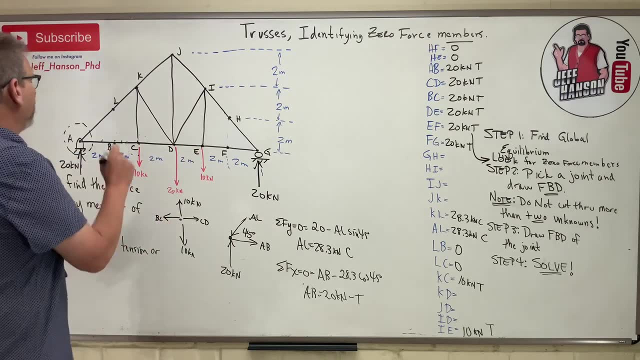 Okay, Man, look how much stuff we just found. Okay, So we got all of this, We got EI down there, So, and it's kind of good to also put check marks on the ones we know. So, we know U, we know U. 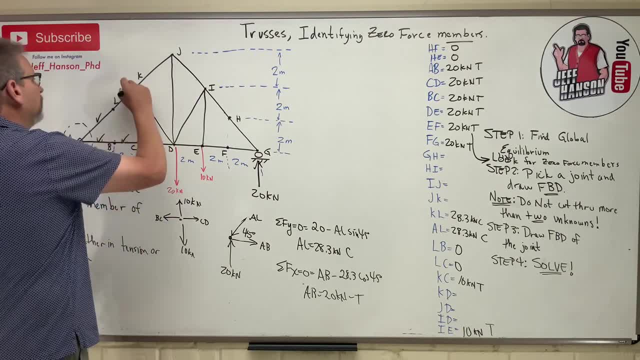 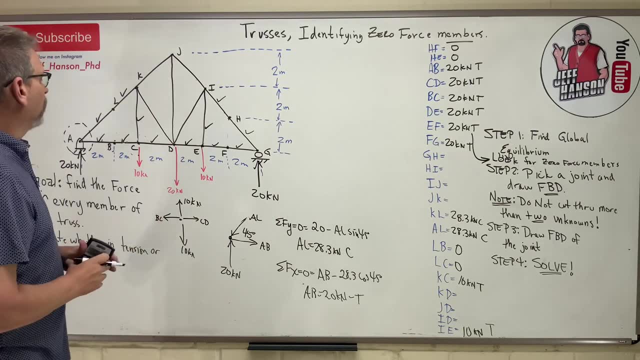 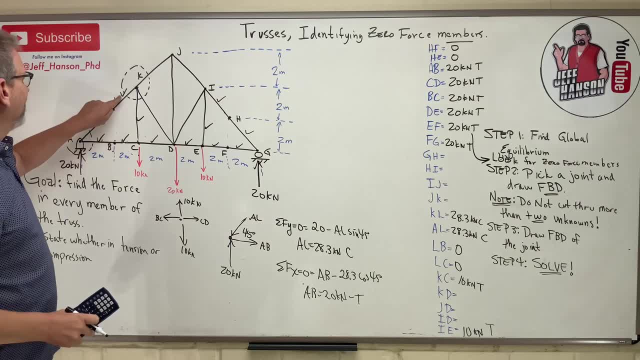 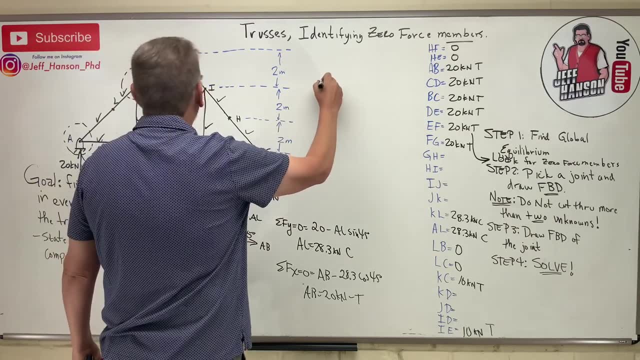 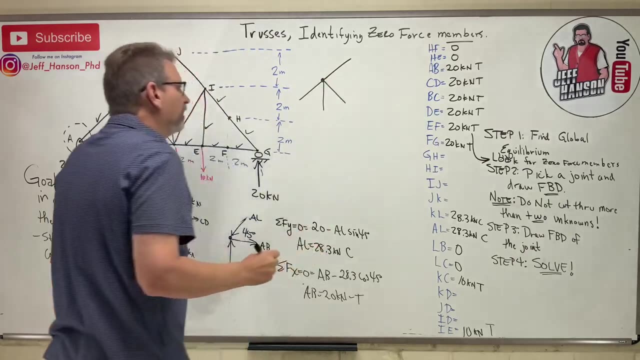 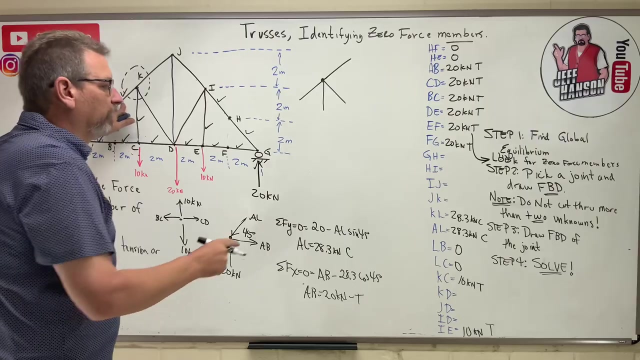 Okay, Joint K. Since I know this guy and that guy, I only have to cut through two unknowns. Okay, All right, So that's going to get me Here's joint K. It's got a one there, one here, one here and one there. Okay, And let's see KL, KL. where'd KL go? Right there. 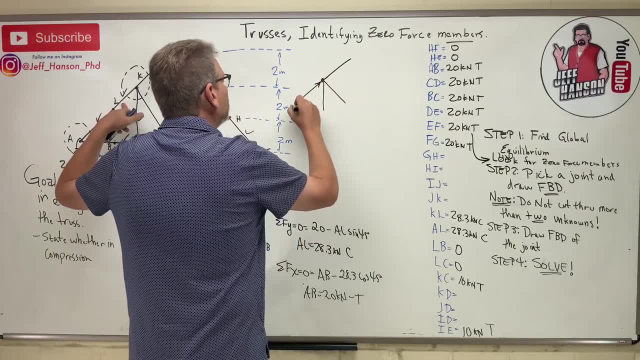 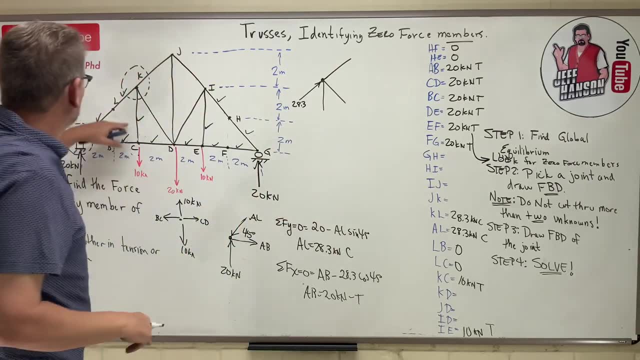 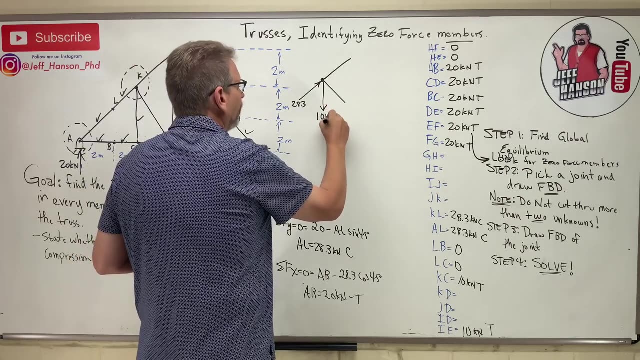 28.3 in compression. So here he is, 28.3.. And then I know this guy which is KC was 10 in tension. Now can I tell about these other ones here? Can I tell which one's up or down, or left or right? 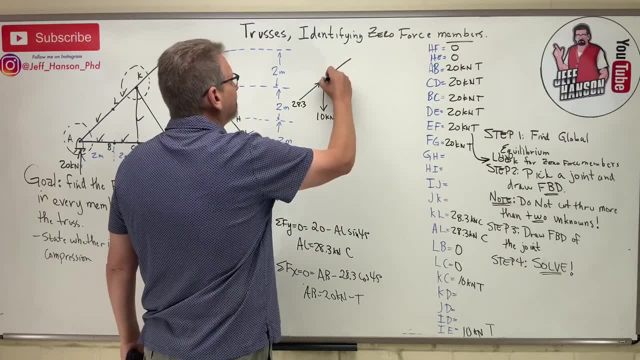 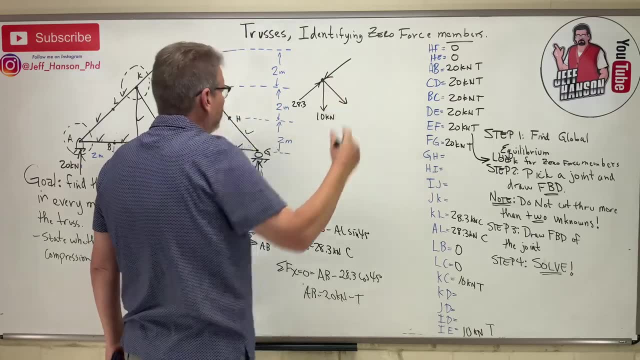 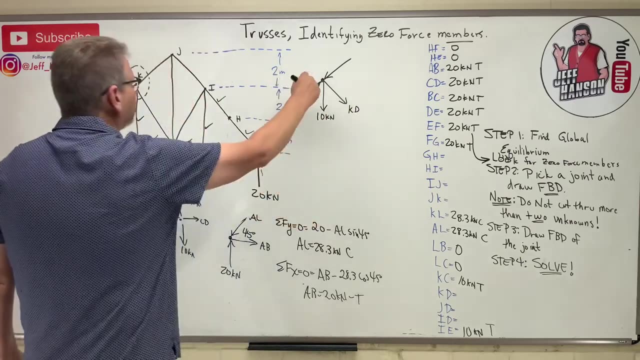 Not really. You know, I kind of think this one's like this and this one I'm not really sure, So I'll just guess him in tension. I don't really know. I think he's probably compression, but I don't know. So here's KD, And this one up here is KJ. All right, And all we need is some. 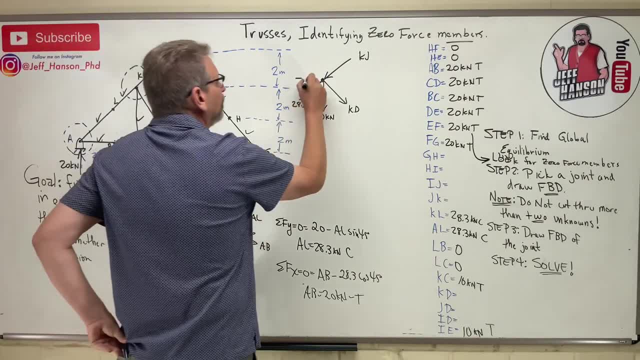 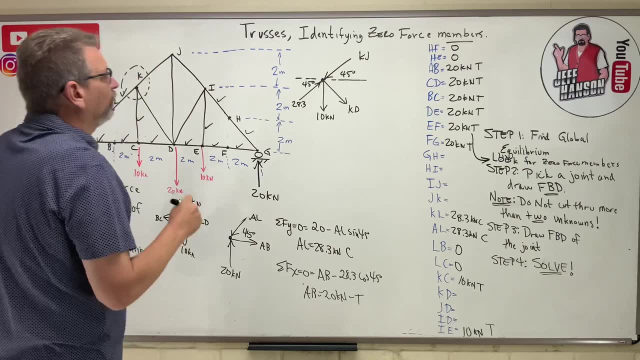 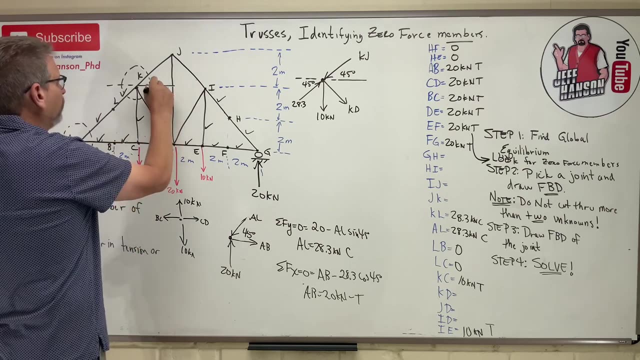 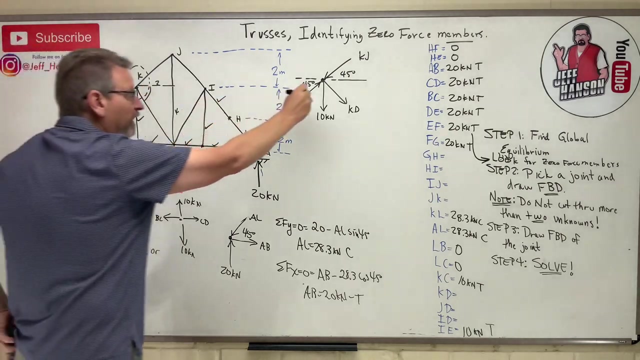 some angles here. Okay, So we know this, we know that's 45 degrees and that's 45 degrees. I don't know that angle in there, Right, But it's two. this triangle right here is two by four. Okay, So this angle right here, which is one I have here that I need right there. 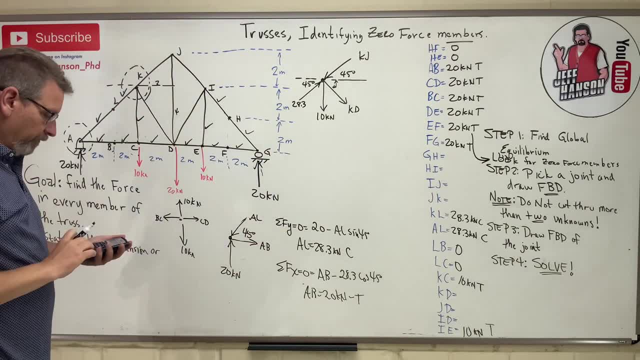 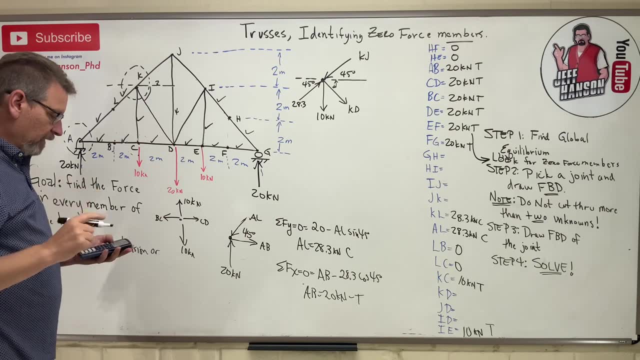 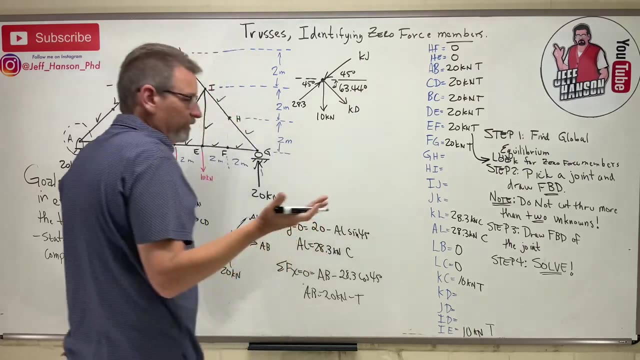 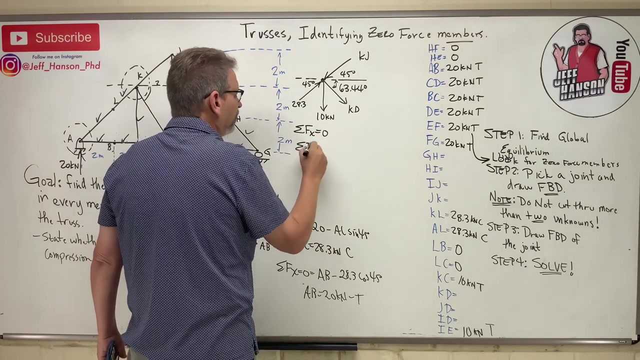 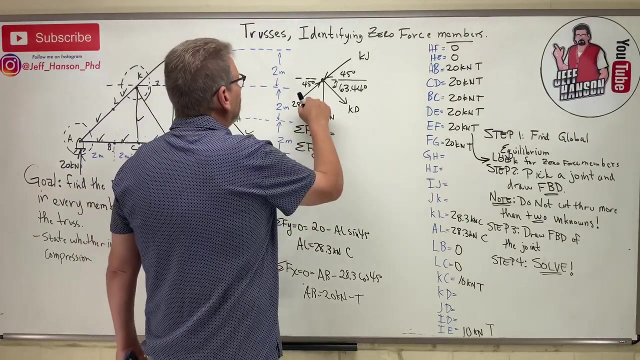 that angle is opposite over adjacent. So four divided by two is two, And so inverse tan of two equals 63.44 degrees. Okay, I'm ready to write my two equations: Some of the forces in the X, some of the forces in the Y. Okay, In the X I've got. what do I have here? 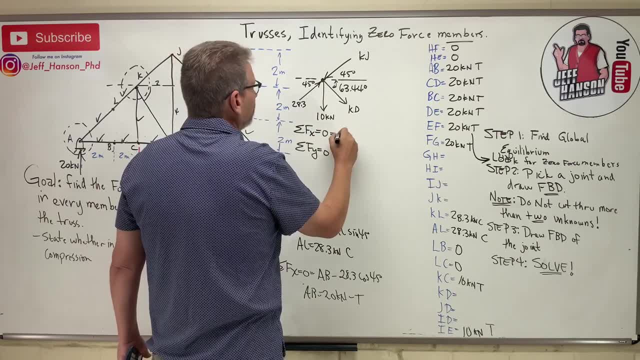 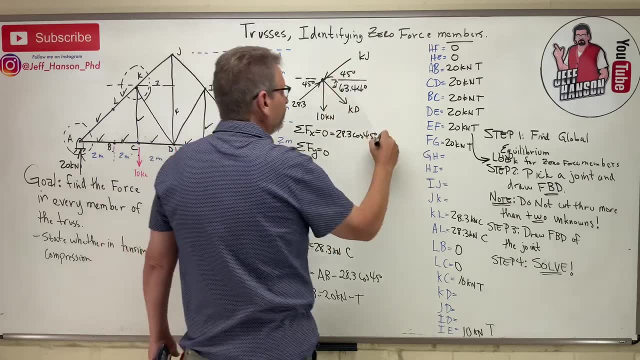 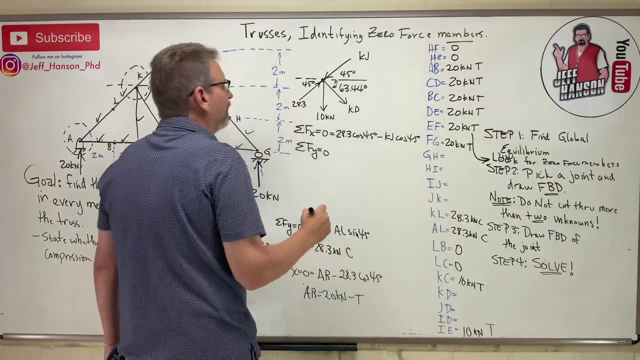 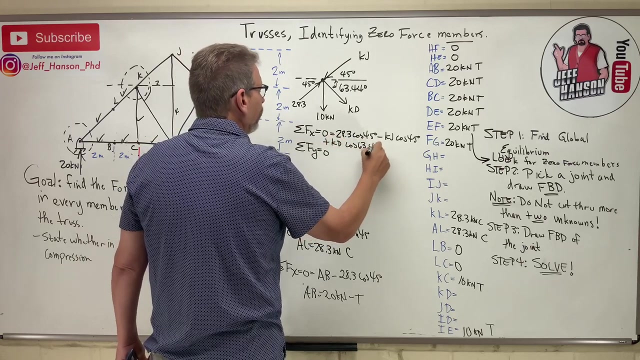 In the X I've got 28.3 cos 45. Okay, I've got minus KJ cos 45. And then I have plus KD cos 63.44.. Okay, So two unknowns in that equation. that's no help, Okay. 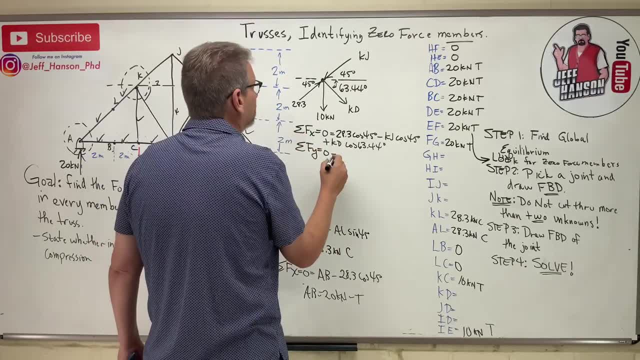 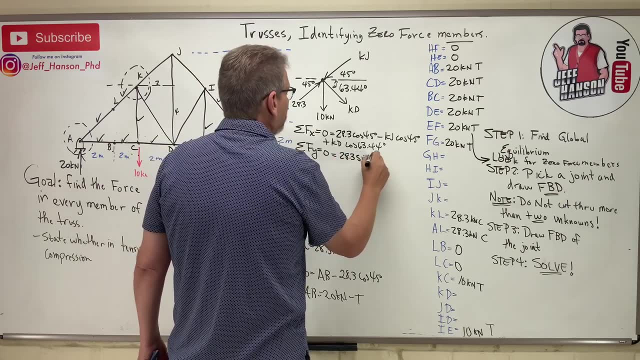 So two unknowns in that equation, that's no help. Okay, So two unknowns in that equation, that's no help. Next equation: I think I'm going to have to use my equation solver to do this- The Y equation. I have 28.3 sine of 45 going up Right. 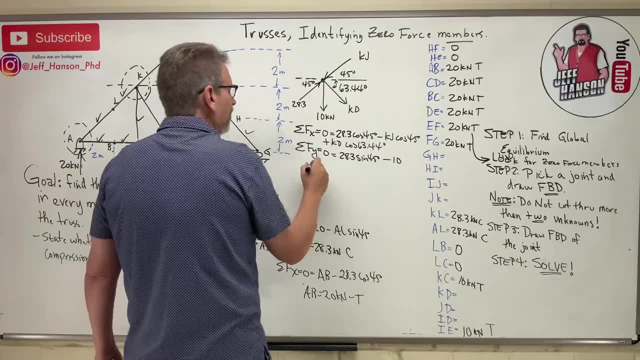 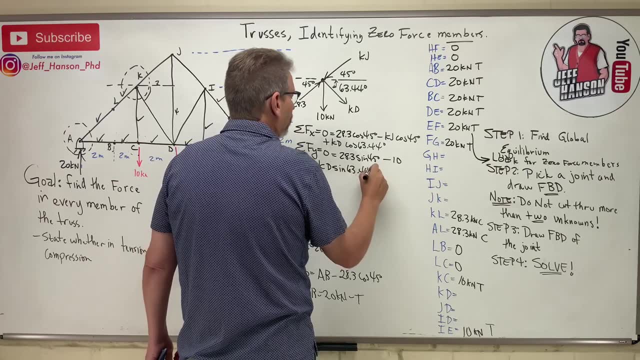 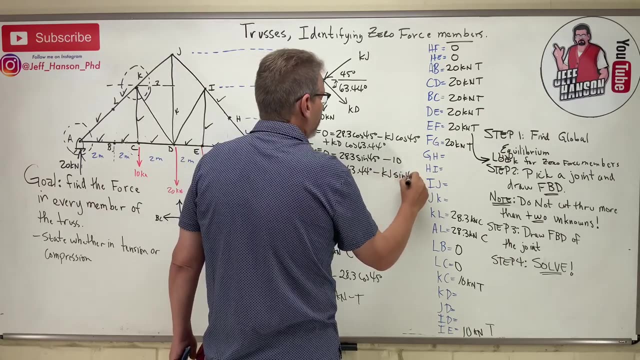 I've got minus 10 going down, I've got minus KD sine 63.44, and I've got minus KJ sine of 45.. okay, so there's my two equations. I'm going to rewrite those where they're a little bit simpler. 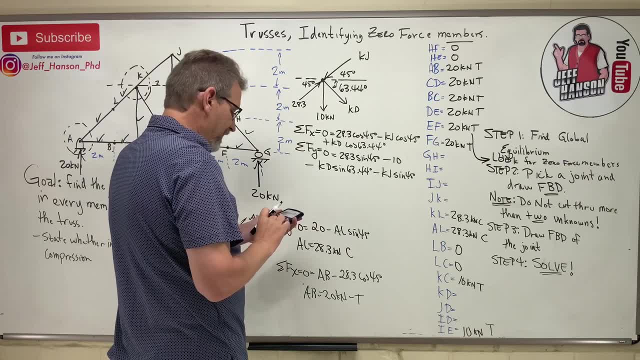 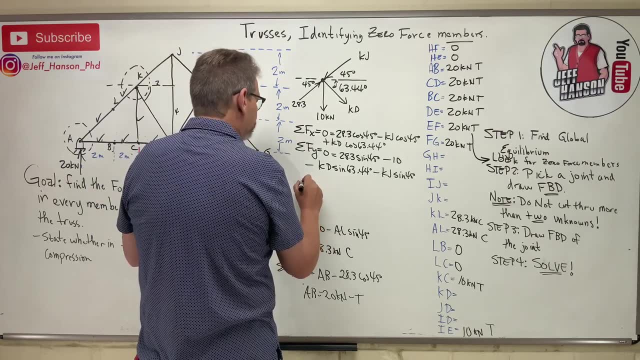 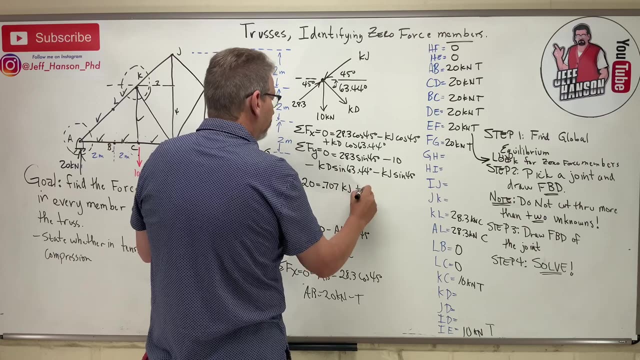 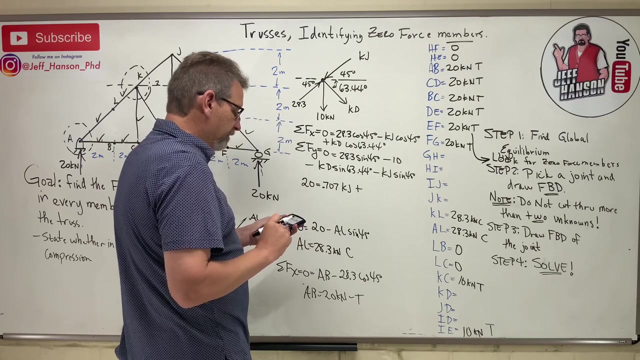 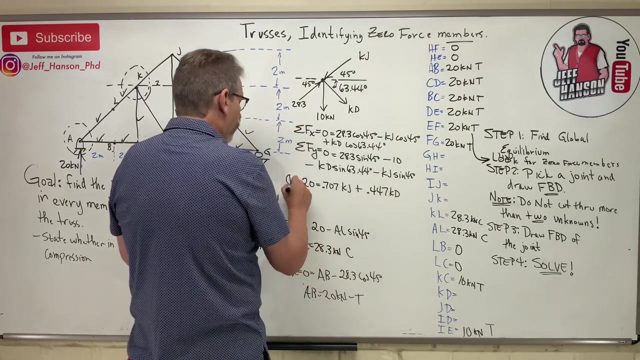 okay, and so 28.3 times cosine 45 is 20. okay, so I have: 20 is equal to 0.707 kj, plus the cosine of 63.44 is 0.447. okay, so there's equation number one. that's from my x equation that's from here. 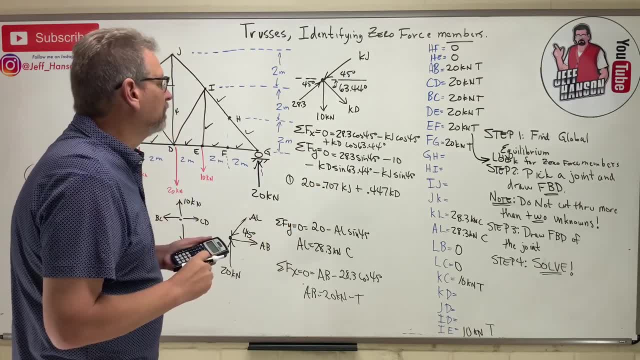 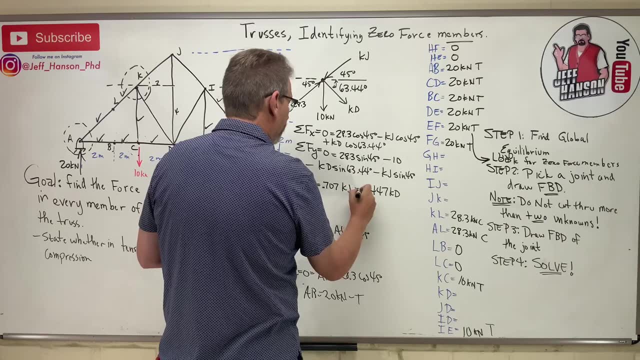 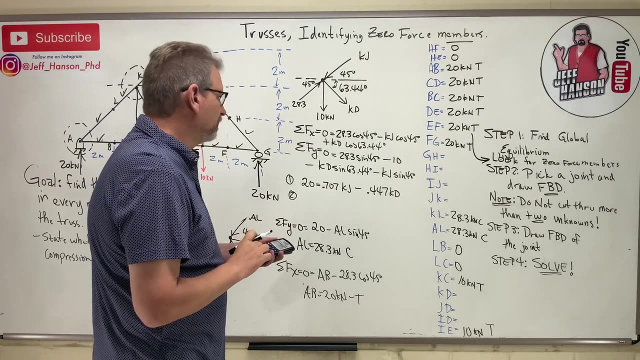 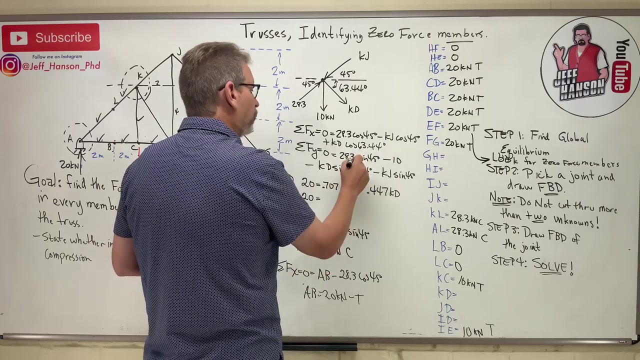 now I'm going to simplify this y equation. okay, oh, oh, oh, I moved that guy to the other side. he became a positive. that guy should be a negative, shouldn't he there? whoo, that was close. okay, equation number two: be careful. algebra 28.3. well, it's the same thing, right? that's 20 is equal to. oh, let's, that's 20 minus. 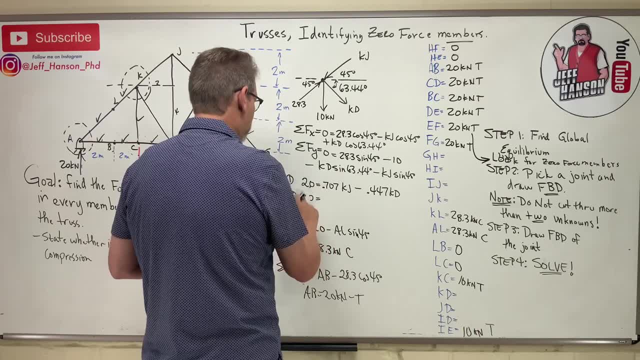 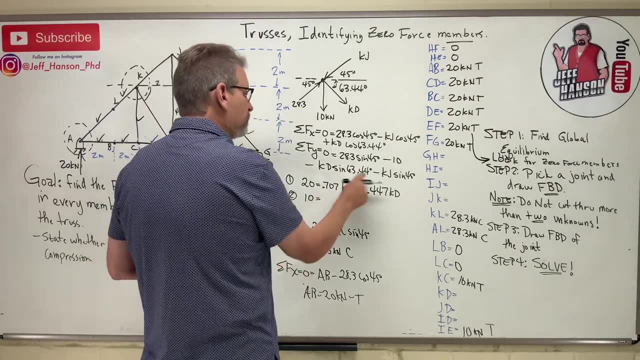 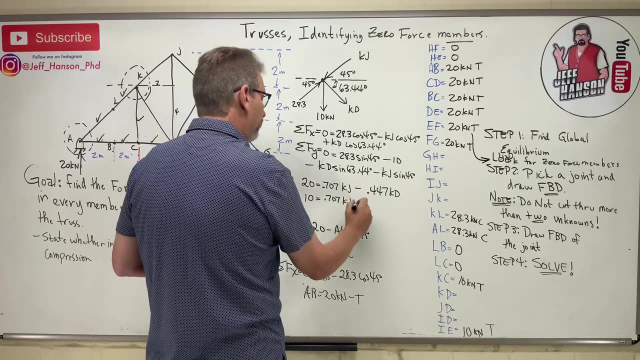 10, right, 20 minus 10 is just 10, isn't it okay? so 10 is equal to: and we got these two guys. I'm going to do kj, which is a 0.707 kj, and then this guy is going to be a plus, plus. 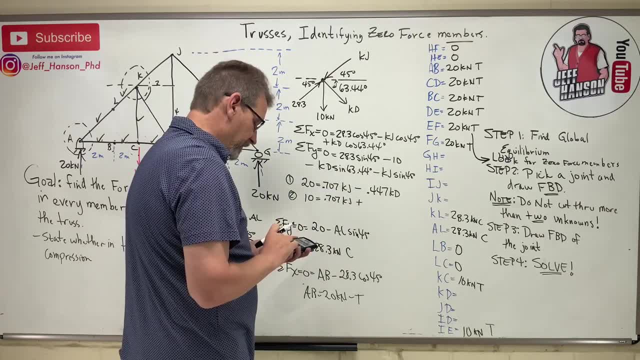 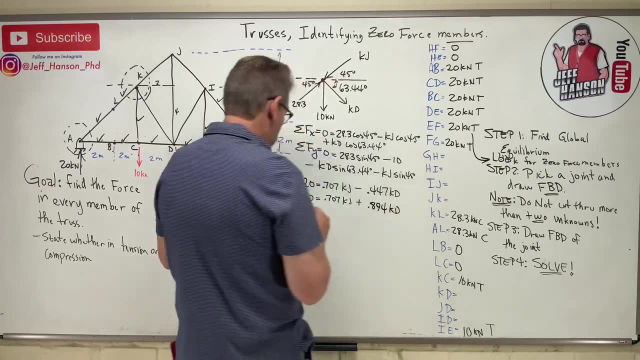 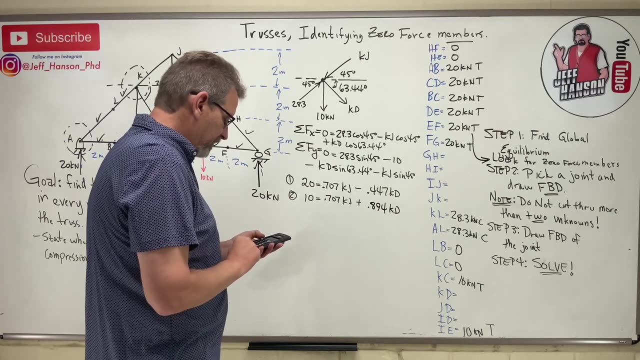 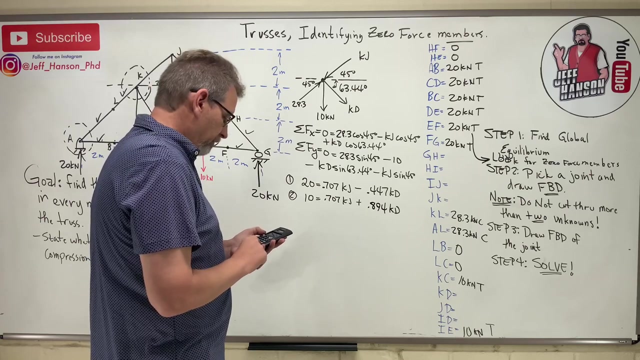 plus, and then this guy is going to be a plus, plus, and then this guy is going to be a plus, plus. sine: 63.44 894 kd. all right, let's throw that in our system solver and let's see what we get for that. okay, so second system: solve two by two: enter 0.707. enter minus 0.447. enter 20 enter. 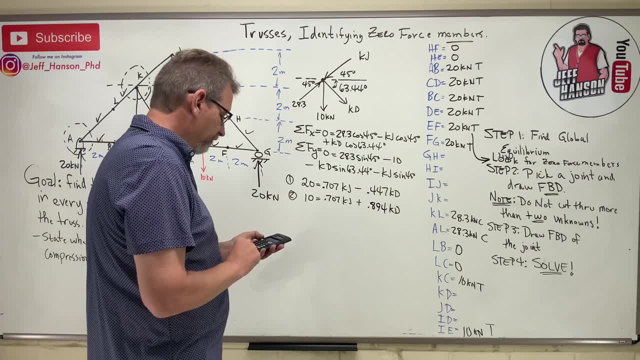 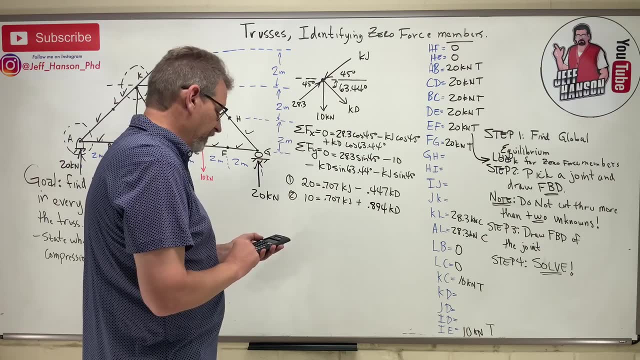 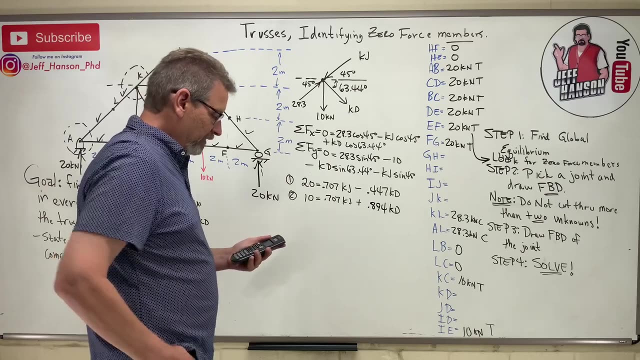 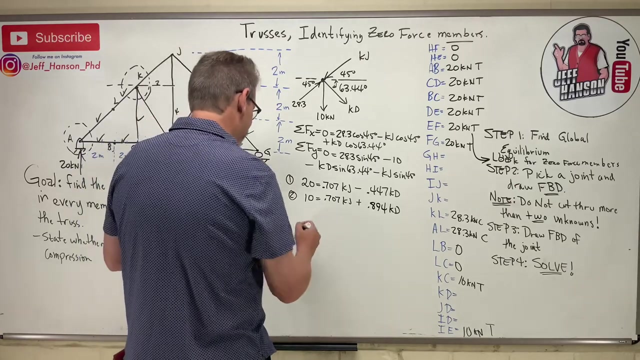 enter 0.707, enter, enter, and then 0.894 enter, and then the last one is 10, enter. if y'all hadn't got one of these calculators, system solver on it, dude- you gotta get one enter. all right, here we go. so here we go. uh-oh, we got a negative. what does that mean? okay, tells me here that kj is equal to 23.57. 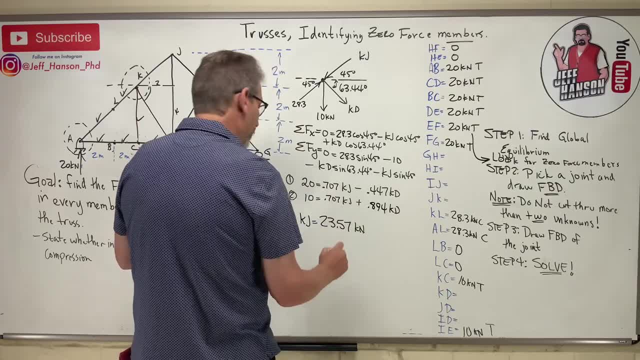 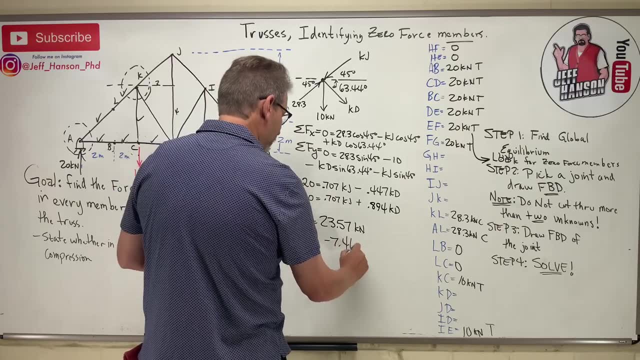 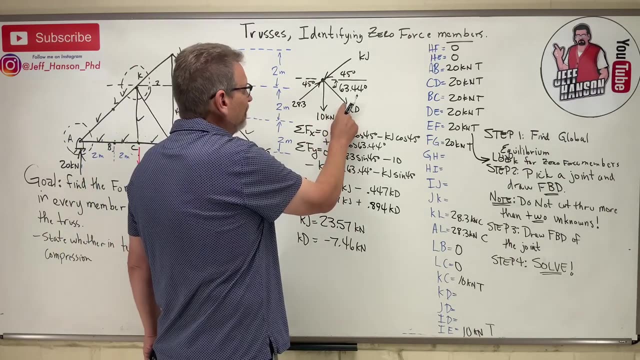 what does that mean? kj is equal to 23.57. what does that mean? kj is equal to 23.57 and kd is equal to negative 7.46. okay, so what does that mean? kd? I didn't know right, I guessed kd. I guessed. 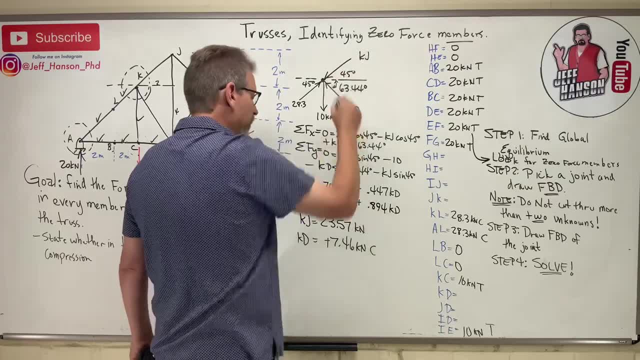 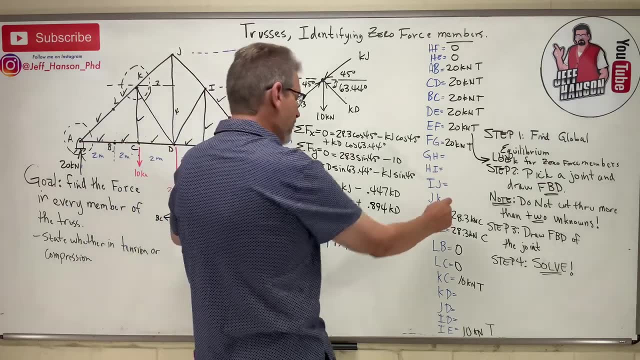 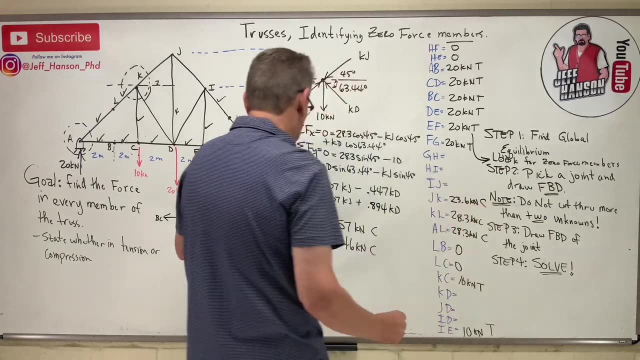 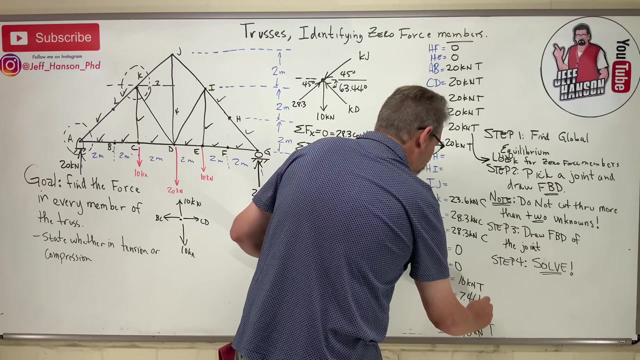 him intention. so what does that mean? he's really in compression. okay, so that guy's in compression. kj going to the joint KJ- KJ 23.6 kilonewtons compression and KD- KD 7.46 kilonewtons compression. 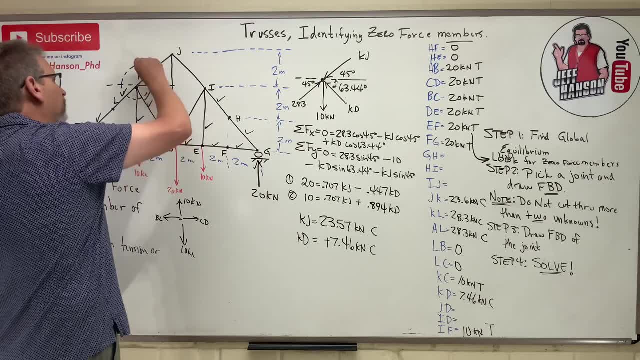 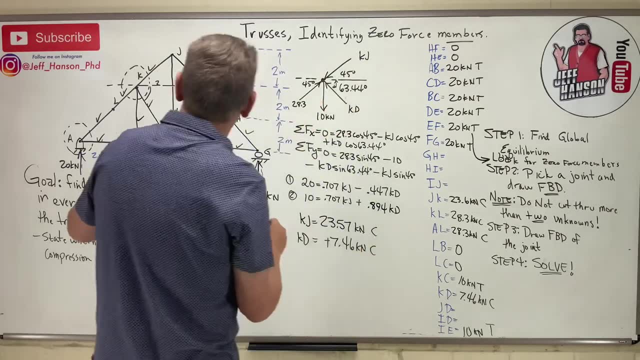 and we also. that means that we found. if I found those two guys, I also found these two guys. so JI and ID, right? so J, let's see. oh no, don't get this wrong: JI is the same as KJ. okay. 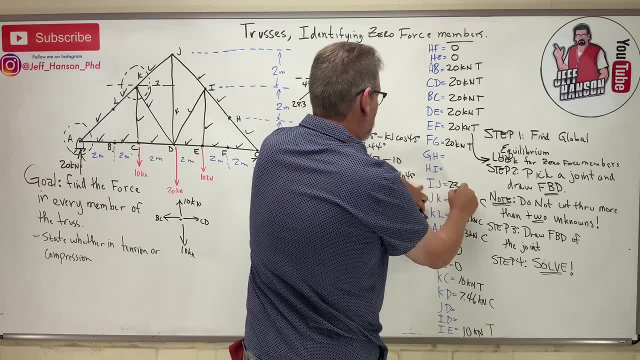 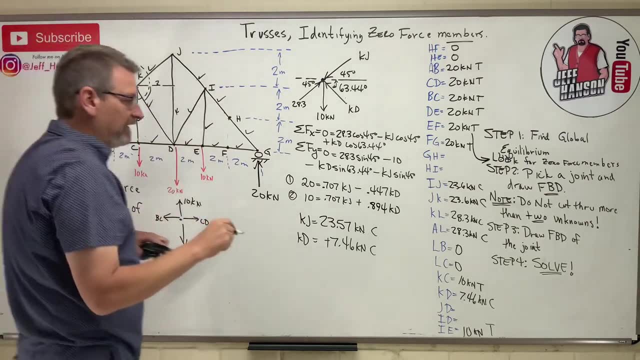 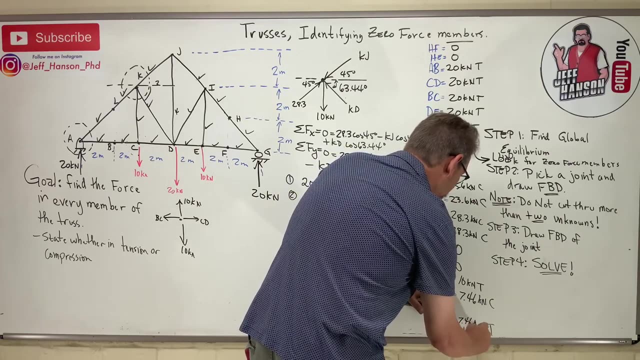 there's JI, there's KJ, so this is 23.6 kilonewtons compression and ID is the same as KD. so there's KD and there's ID, so 7.46 kilonewtons compression. 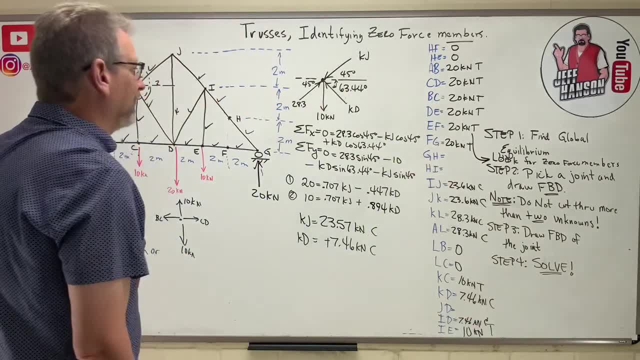 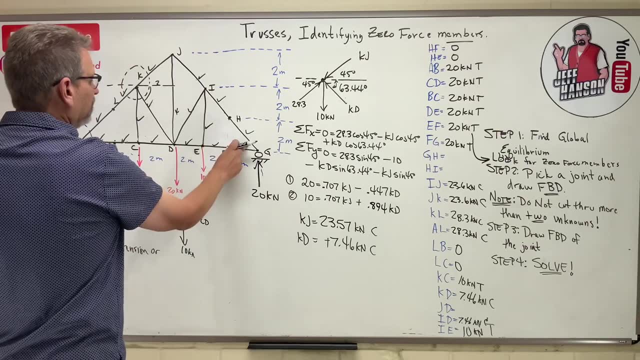 Okay. so what are we left with here? what are we left with GH? where is GH? A, B, C, D? oh, I know, GH, don't I? GH was the same as AL, so GH and AL are the same. 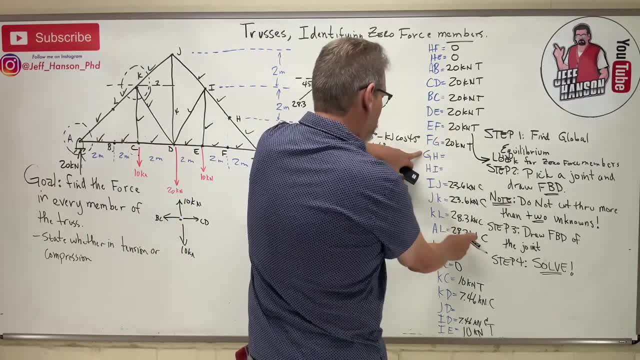 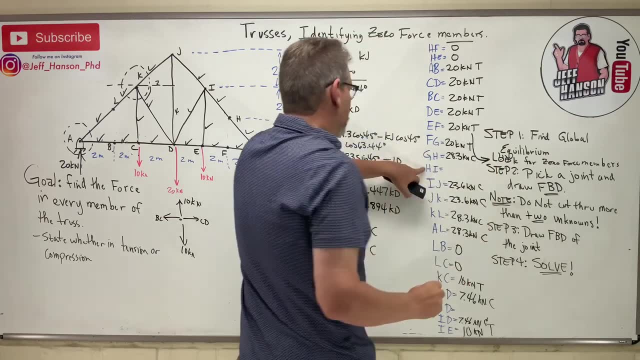 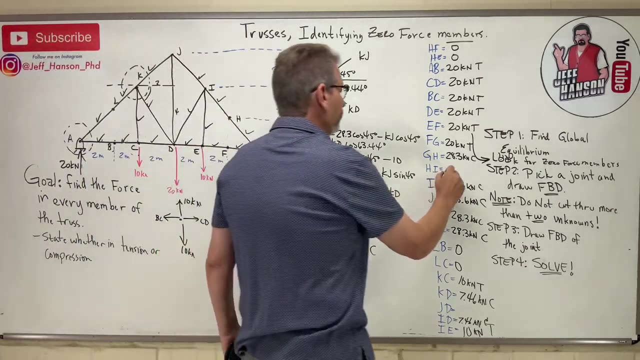 where is AL AL, right there? 28.3 compression- compression. and then HI. where is HI, H, HI. oh, that's the same thing, isn't it? HI also 28.3 kilonewtons compression. okay, 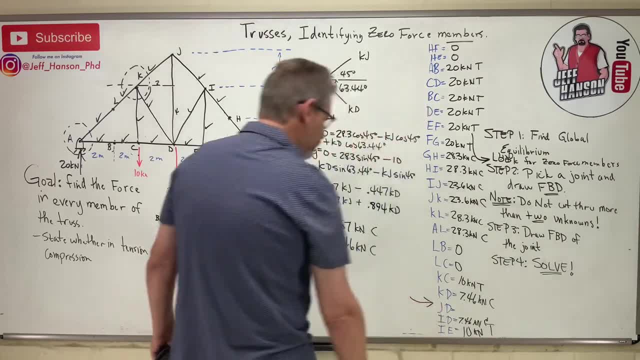 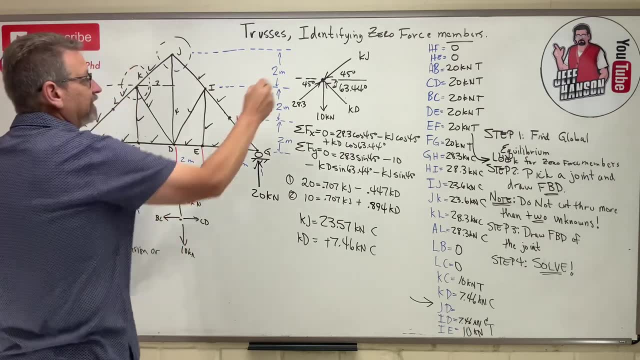 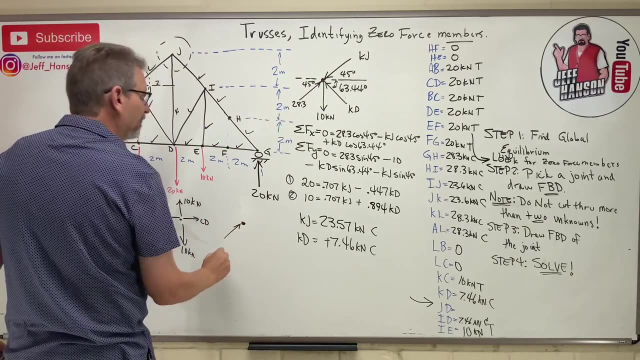 and who does that leave? it leaves one dude right there, JD. we could come back with this last guy right there, right, and we get KJ was in compression. so on the other end, he's going to be in compression. so here's joint J. I've got this and that guy was KJ. was how big was KJ? 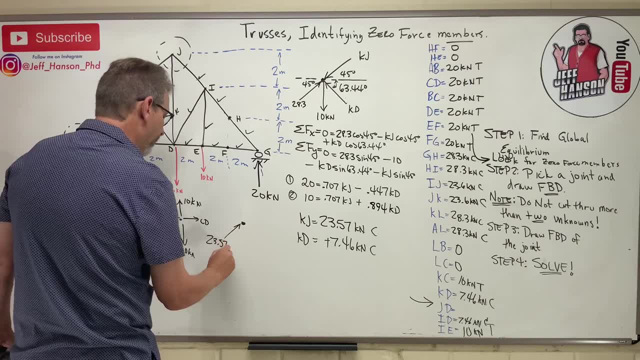 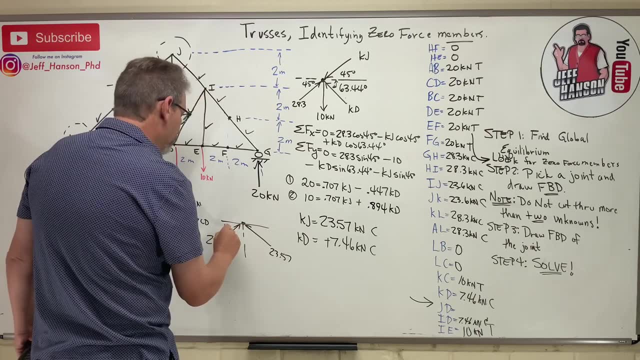 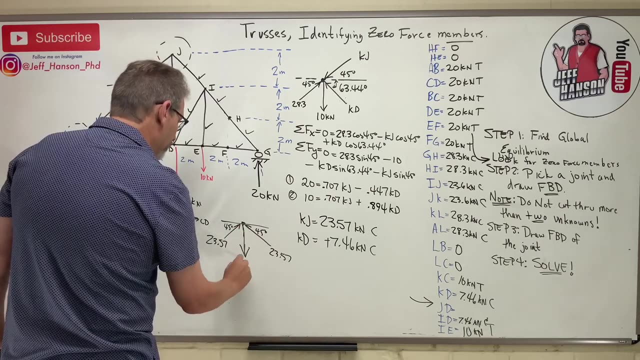 23.57, and then there's the other one, 23.57, and these are 45 degrees, 45 degrees. and then there's JD right here, up up. JD's got to go down, doesn't he? JD? sum of the forces in the Y. 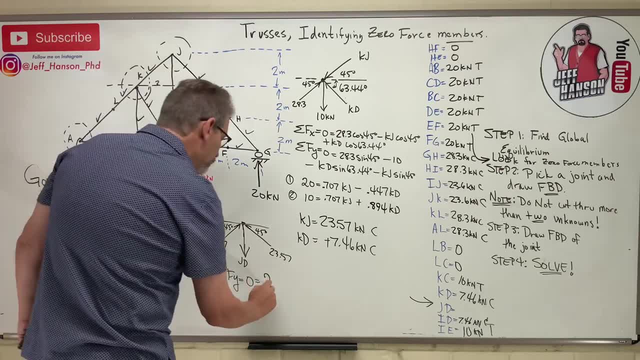 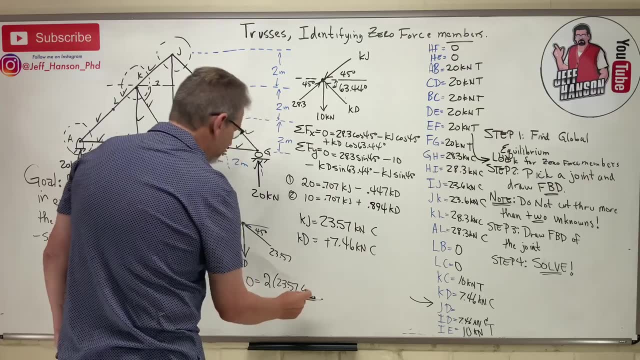 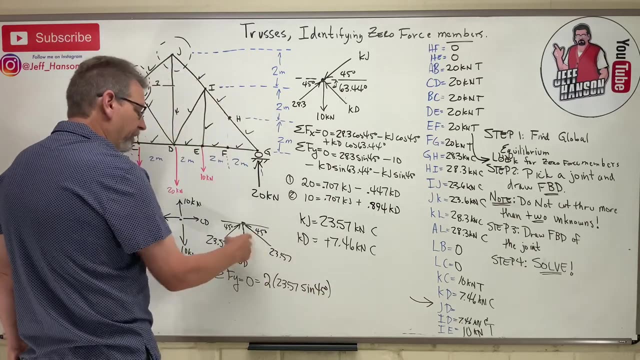 is equal to zero, is equal to two times 23.57 cosine. well, really sine, but it doesn't matter. same thing. sine 45, right, that's these two guys going uphill, their components minus JD. so JD is going to be in tension and it's going to be. 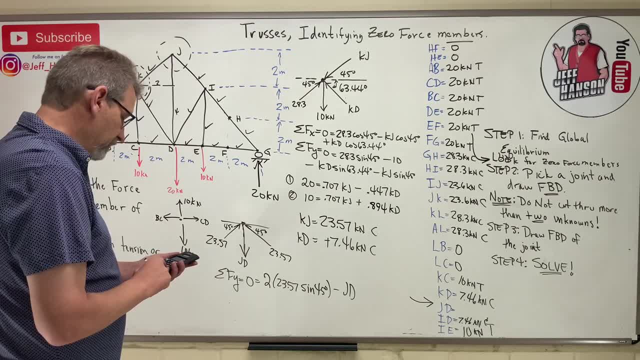 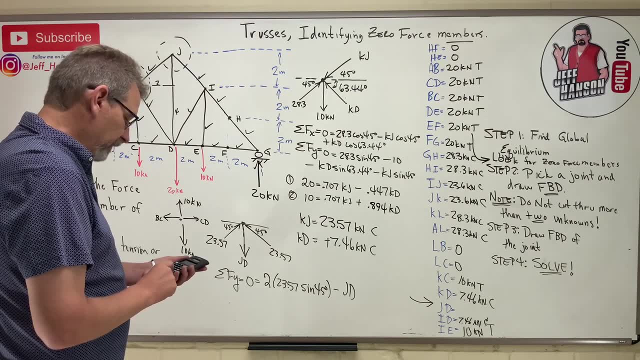 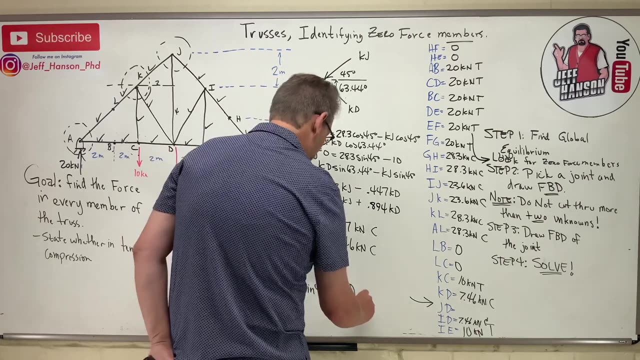 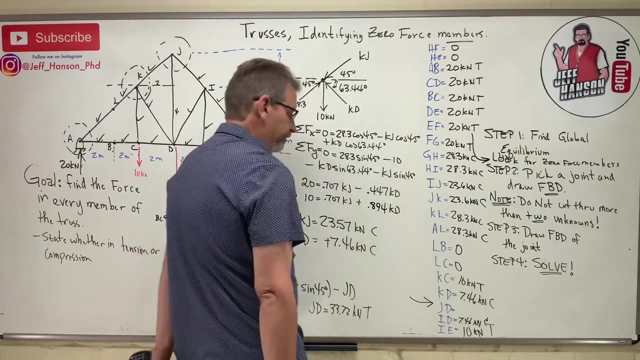 two times clear, clear two times 23.57. equals times 0.707, equals 35.. 33.32, so JD equals 33.32 kilonewtons in tension. that's the last one, 33.32 kilonewtons in tension. 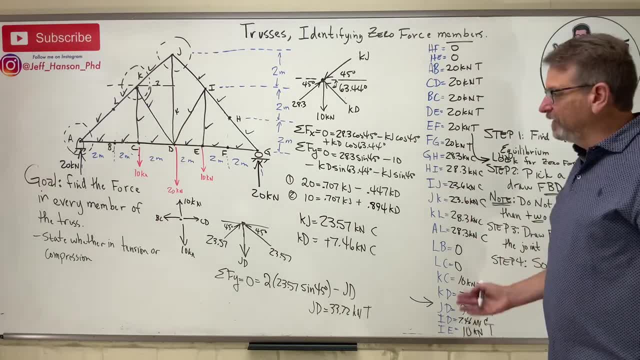 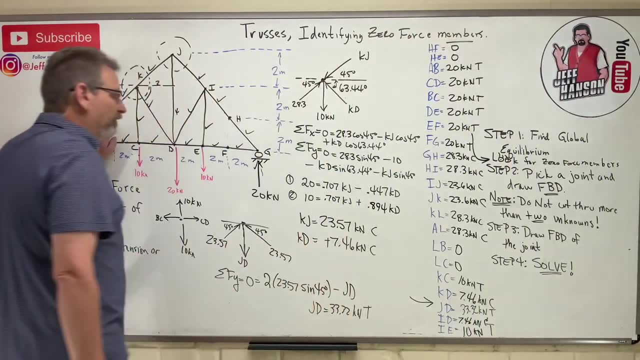 bam. look at, that was daunting, wasn't it? but it wasn't that bad dude, we are so smart, okay, identifying those zero force members helps us. now here's the secret, okay, if you miss it, 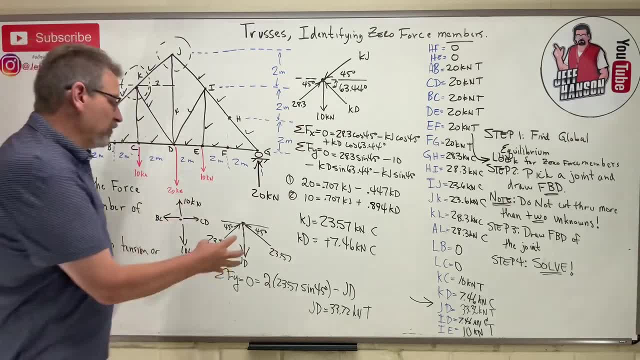 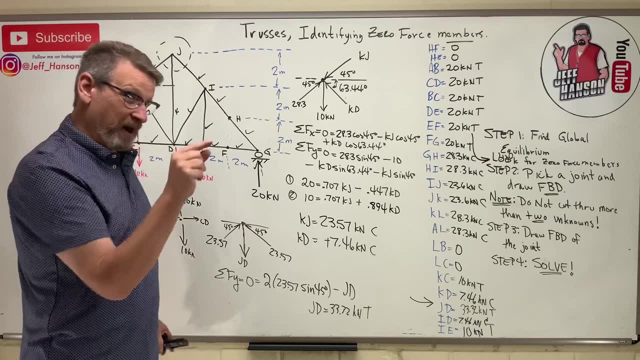 you're like, I didn't see it. I didn't see the zero force member. well, when you do this, when you do your little method of joints, you'll still get zero. okay, it just saves you a little bit of time if you can spot them. that's all it does. you'll still get zero when you do the math.